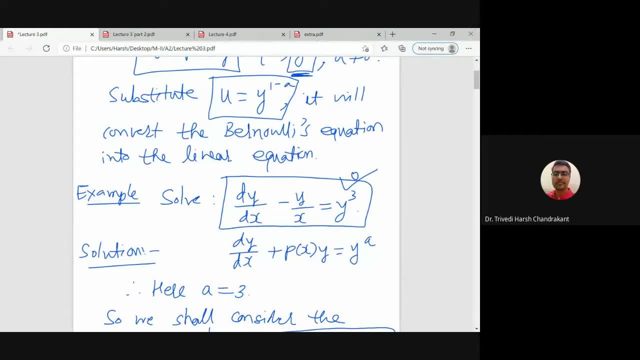 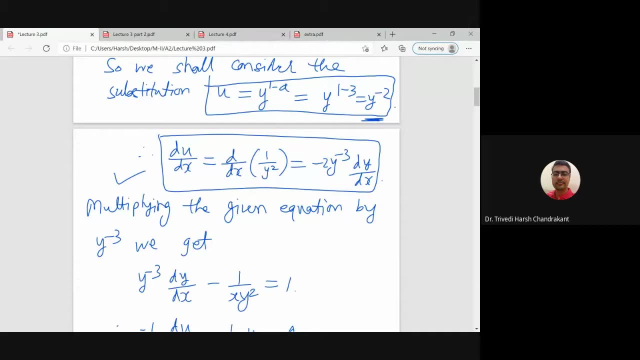 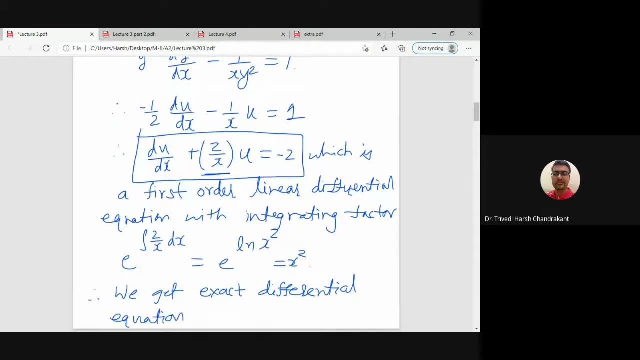 example of that. so whenever such a example is given, we will use the substitution method. and by substituting u is equals to y power 1 minus a, we can see that we can convert this differential equation into first order linear differential equation. and then we know what? 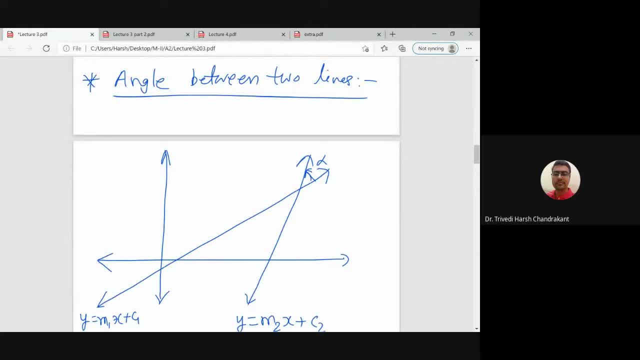 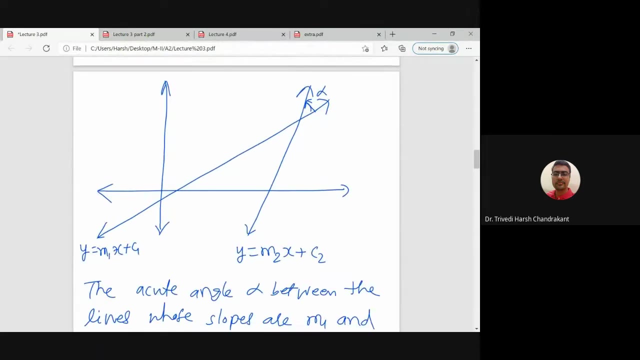 is the how to solve first order linear differential equation and finally to get the final solution. we substitute the first order linear differential equation And then we substitute that function u once again and then later on we discuss this angle between two lines. so here we can see that whenever we consider this line, y is equals. 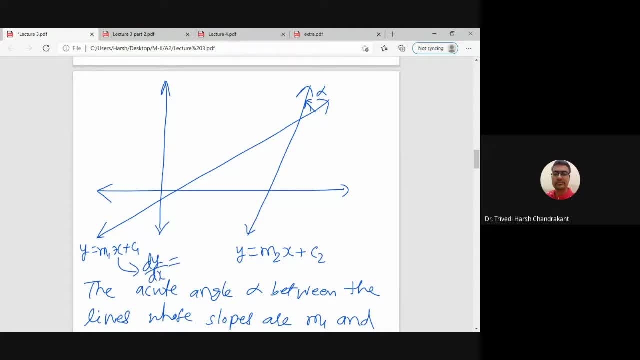 to m, x plus z. it is, when we convert it into, divided by dx, equals to f of x- y. we basically get this equals to m1, and m1 is nothing but y minus p1, minus p2 and p3. So in this case we get a standard function. 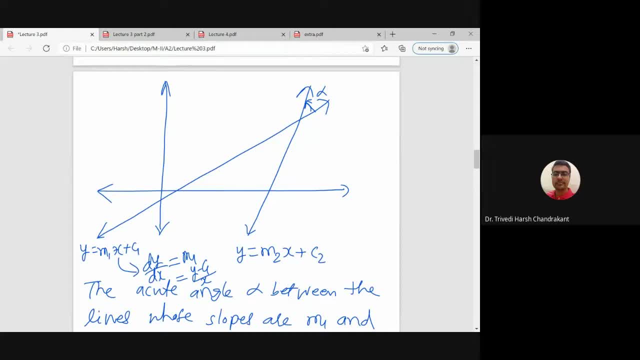 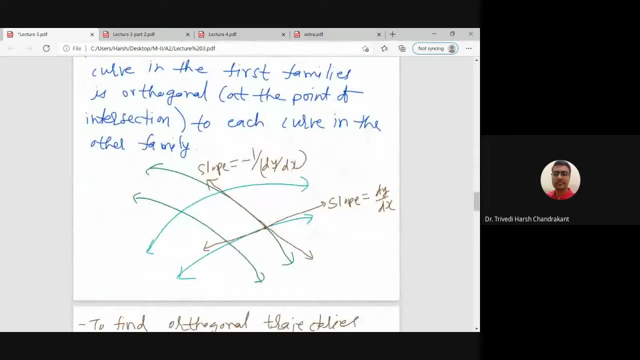 by X, right? so this is a function of X and Y, which is nothing but M, 1 in this case, whenever the curve is line. so this idea has been generalized here for the orthogonal trajectories. so this slope is divided by DX, but there is nothing but the Pope X, Y, and then we take the inverse of the slope. that means 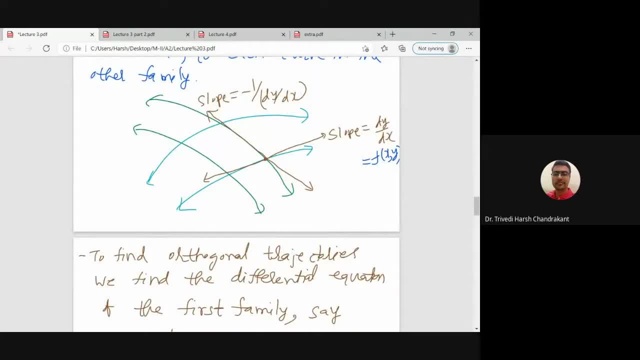 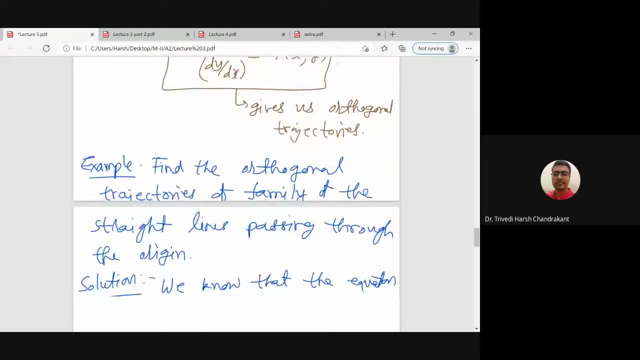 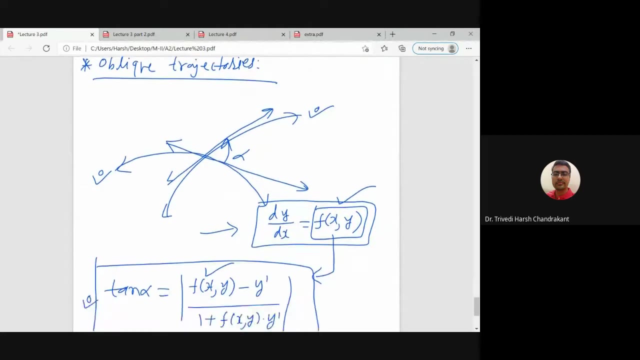 basically, we consider minus 1 upon y dash equals to f of X, Y, and the same idea is used for the orthogonal trajectory, also, for the oblique trajectories also. so first curve, we convert, we first find out its differential equation. we write in this form: you have a DX equals to f of X, Y. 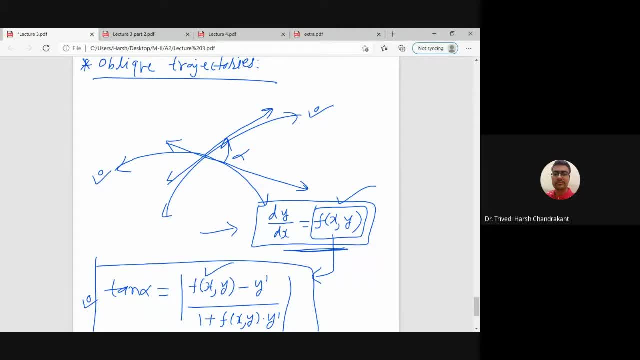 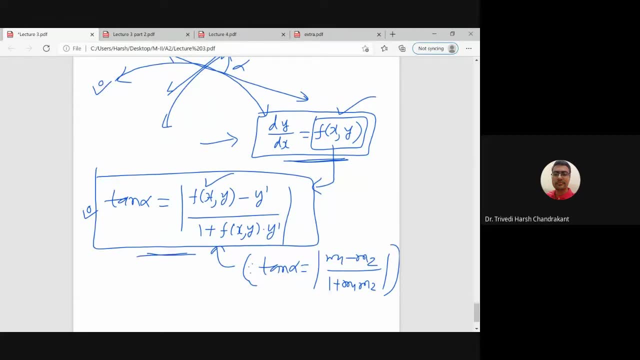 and then whatever F we get. you can write in this form: you have a DX equals to f of X, Y, and then whatever F we get from the first curve that we substitute in this equation of the angle formula between with the slopes. so this idea we use here, using the differential equation. 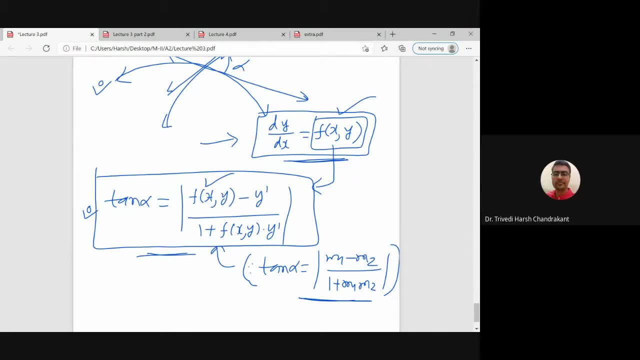 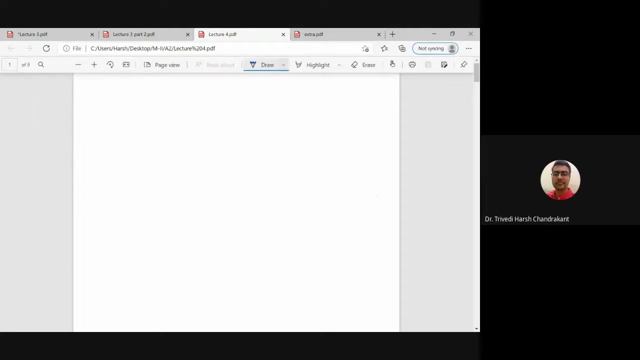 so that we get the differential equation of the second curve of the oblique trajectory and then we solve that so we get the all the curves in the oblique trajectories. so that is essentially what we what we have discussed in the previous lecture. today we want to discuss initial value problems. 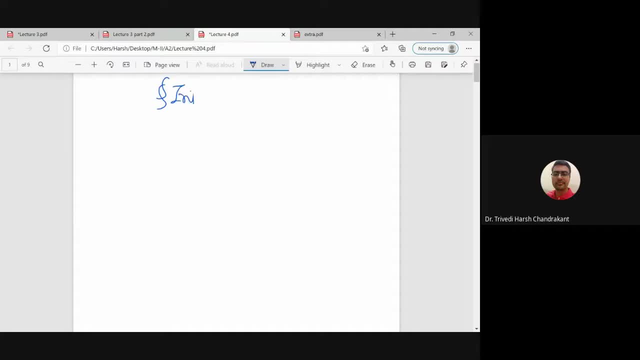 so what are the initial value problems? so essentially, uh, so far in the differential equation part, our goal was to study the equation: dy by dx equals to f of x, y. that is the given differential equation and we want to find its solution right. that is the main. 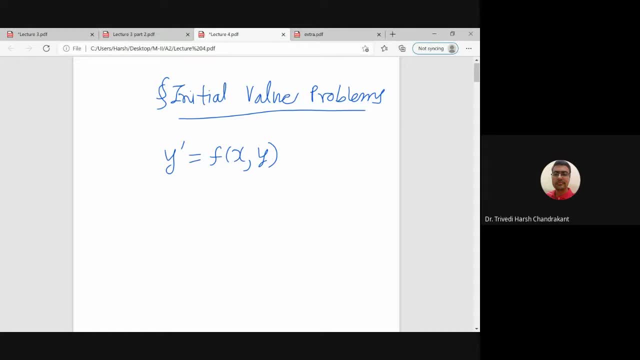 question. so we studied several methods to find solution of the such equations. so if such equation is of the form separable variable form, or or it is linear differential equation, or it is Bernoulli equation, or it is exact differential equation, or it is integrating factor method. 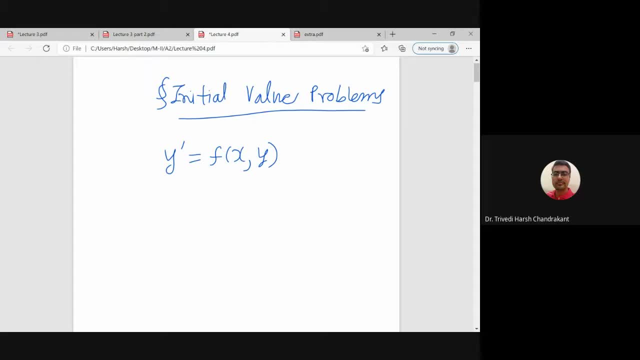 in such a if the given differential equation is either of this form, we know how to solve it. but if the given differential equation is not of this form, that means it is not exact, it is not linear differential equation, it is not Bernoulli type equation. then, in general, how will solve this? 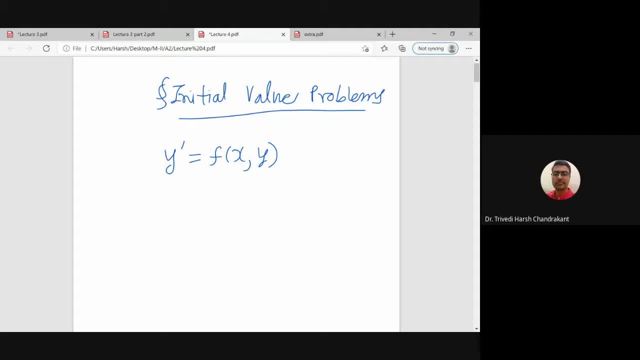 equation. so there are two questions associated with this. so first thing is whether, if such a equation is of this form, then how can we solve the question in this way? so the first question is given, whether it has a solution. that is first question. second question is if. 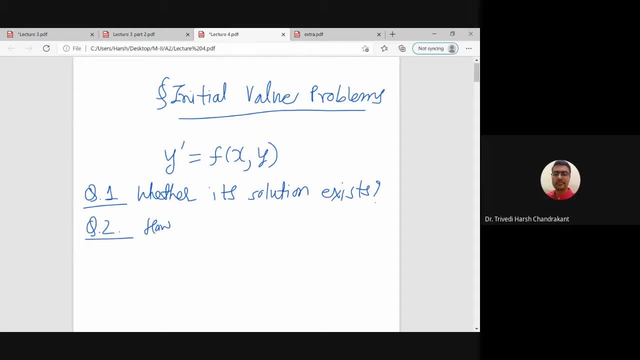 such a solution exists, then how to find it, how to find the solution right? so this is the question which we are exploring in this. so far, whatever we have seen the matters, to answer these two questions based on what differential equation is given, what type of differential person? 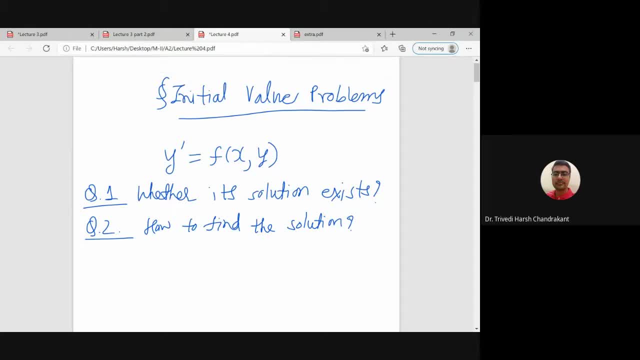 but in general, is there any matter which works for all the problems? so answer is no. there is no any particular method. so that's why we studied several methods, but there is a common approach which works in some of these methods as well as other methods. so that means there is a partial answer, partial answer of both these two. 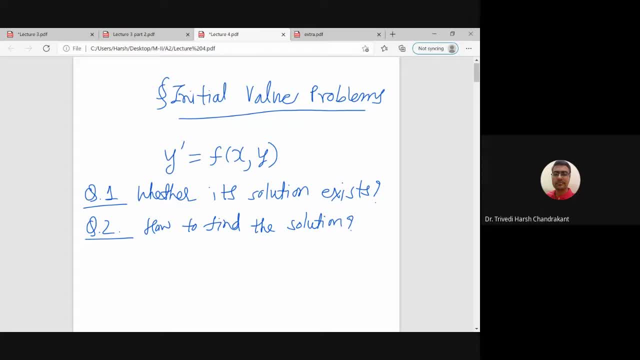 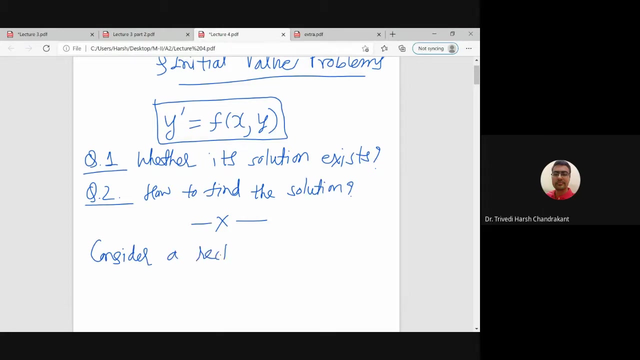 questions, and that is the method of initial value problem. so initial value problems will be. that means we will consider such a differential equation with some extra conditions on the function F, right? so let us start with posing those conditions. so the first thing is consider a rectangle. so this rectangle is defined as a rectangle. 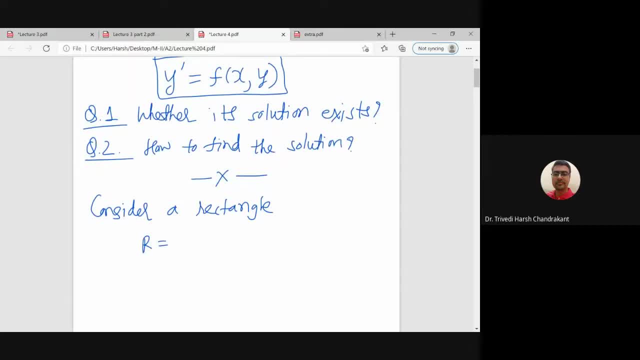 so this rectangle is defined as a rectangle. so this rectangle is defined as a rectangle. find, as r is equals to points xy in the xy plane, such that x belongs to the closed interval, x minus x, naught minus a to x, naught plus a and y belongs to the closed interval. 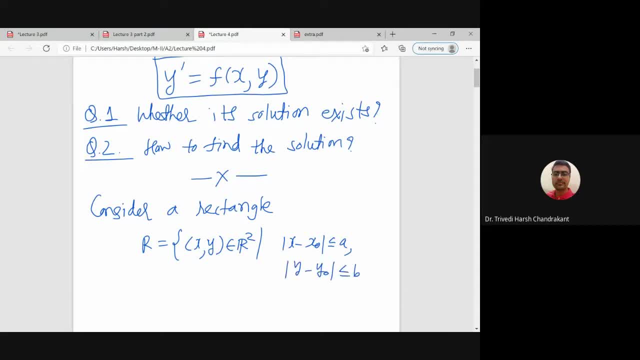 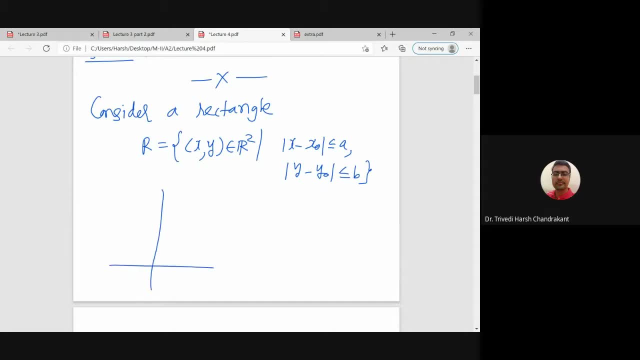 y naught minus b to y naught plus b. so this rectangular, we know what is the diagram, we can easily draw this. so our point is: x naught is here. let us say then: is x naught minus a, x naught minus b. of course, here a and b are positive numbers. 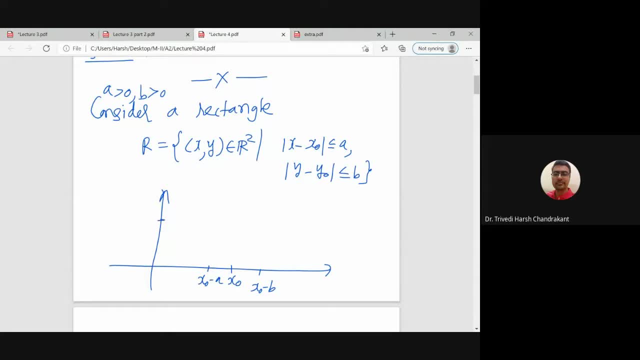 right, and suppose our point y naught is here, then this is y naught minus b and y naught plus b, so that means our rectangle is essentially this part right. so that is this rectangle r, and in this rectangle we have this point: x naught, y naught. 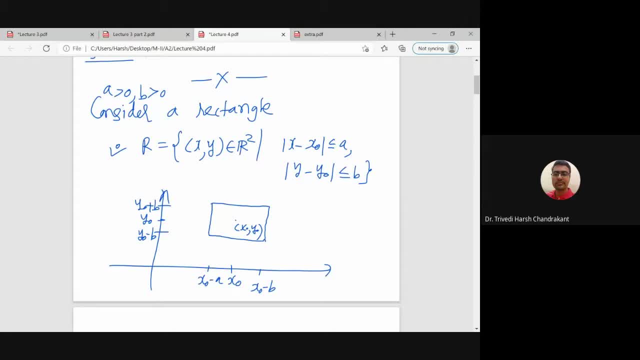 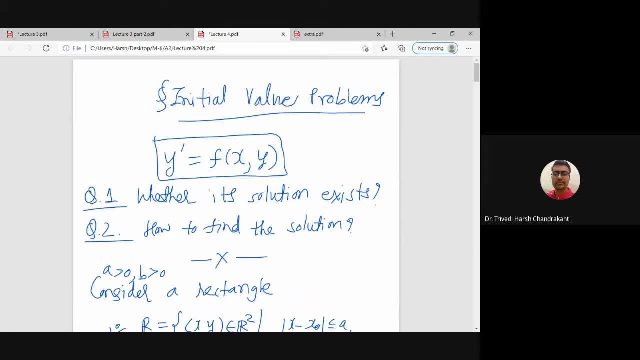 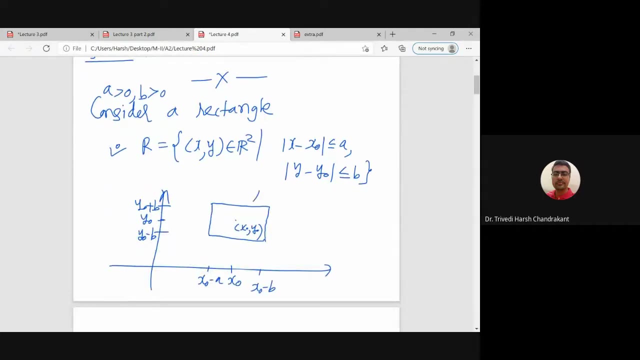 so what we will first, what we want is we are given this differential equation: d y by d x equals to f of x, y, and we want to find a curve, y, x, which is solution of this differential equation, and it passes through the point x naught, y, naught. 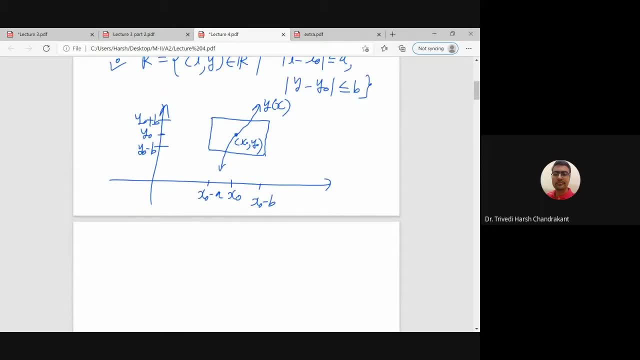 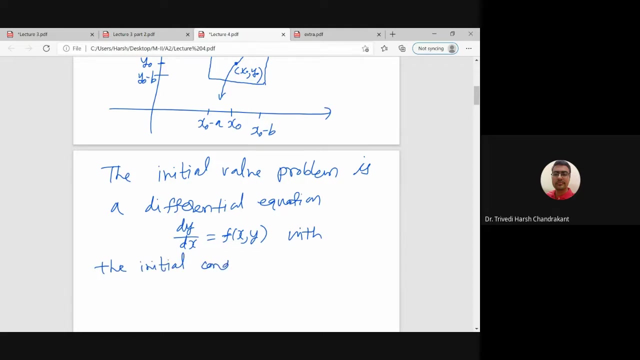 so that means what that means. yeah, so that means the initial value problem. so the initial value problem is a differential equation: d y by d x is equals to f of x y. the essequ appear in coordination with special condition, with some initial condition, with the initial condition. 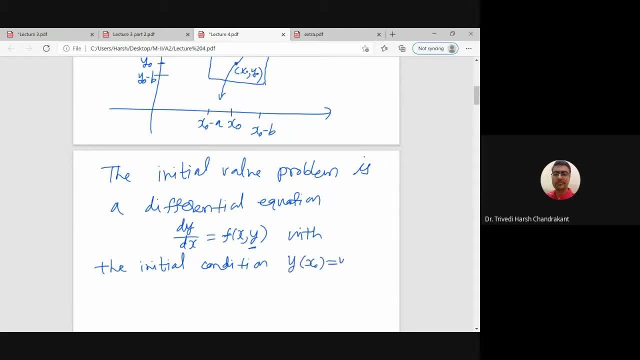 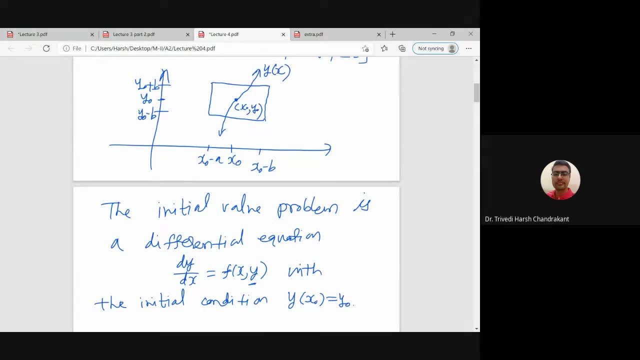 that y said is this: function y, which is a function of x that satisfies it, passes through x naught, y naught. so that means y of x naught is y naught right. y is a function of x, x, x variable. so the goal here is to find the function y. 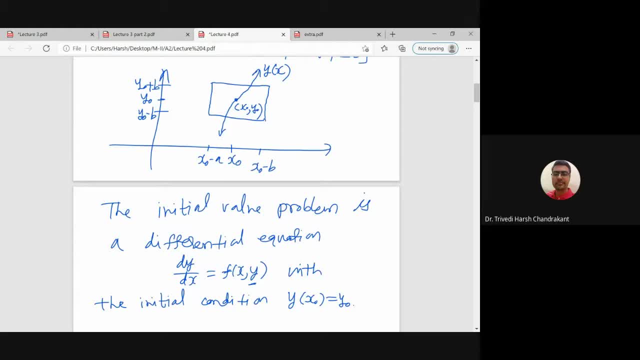 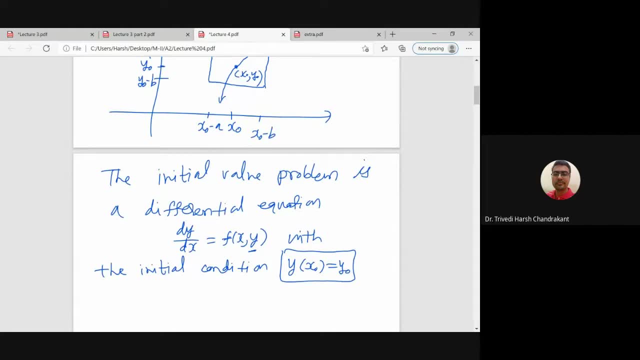 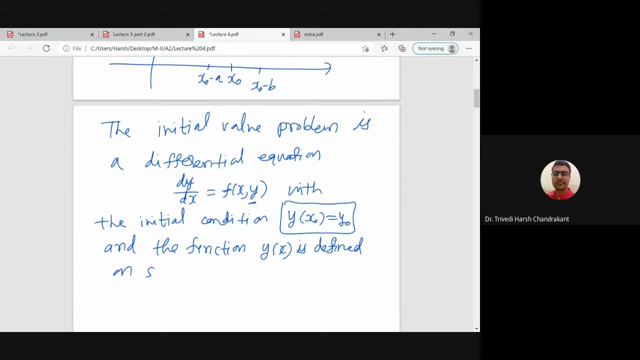 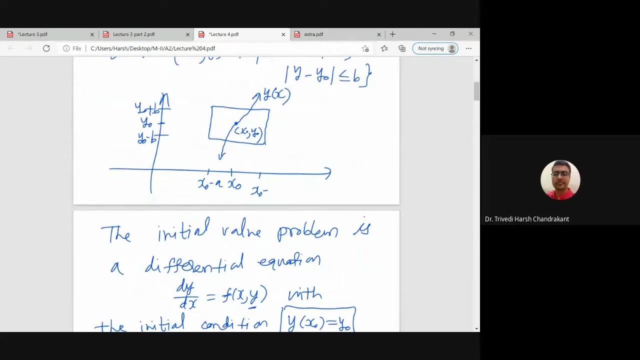 which satisfies this differential equation and it also satisfies this initial condition. so this condition is known as initial condition, that whenever we apply y on x naught, we get the value y naught right and the function yx is defined on some interval i right. so clearly, i is a subset of the interval x naught minus a to. 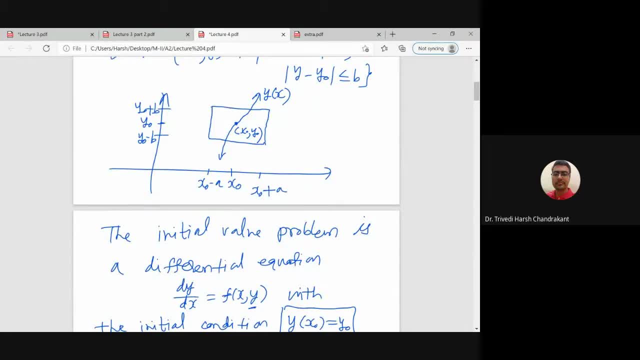 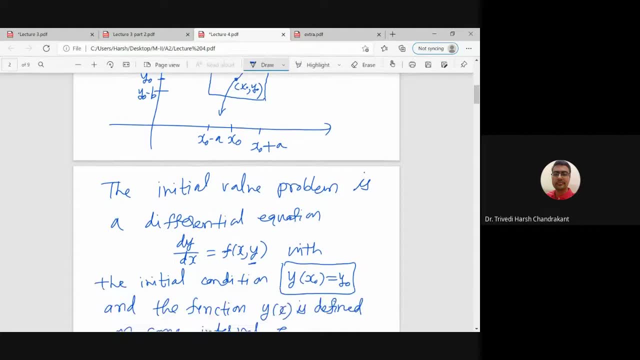 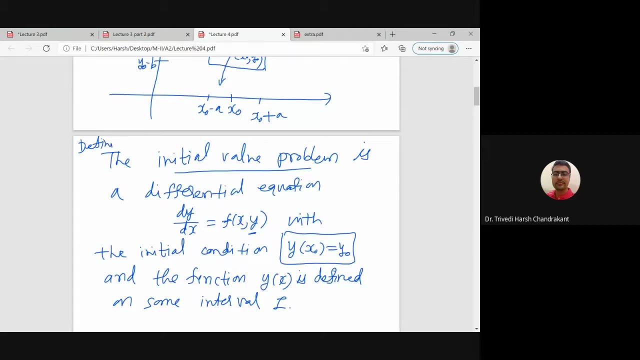 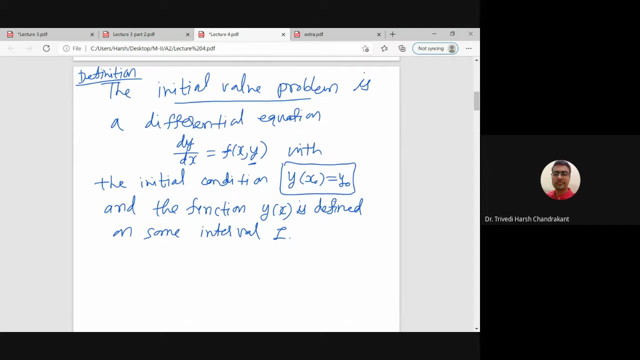 x naught plus a right. so these are the typo, so it should be x naught plus a. yeah, so to solve such an initial value problem. so this is definition of initial value problem. what condition we will require on the function f? so first condition which we will impose on the function f is that the function f 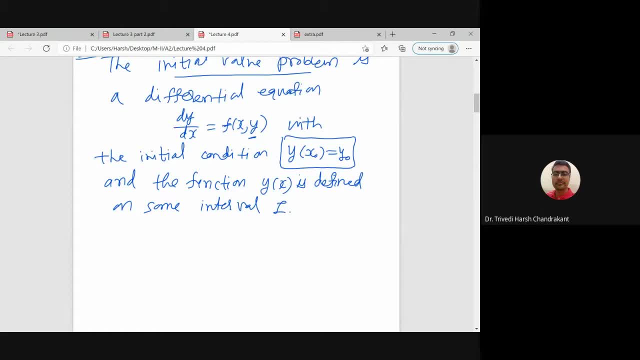 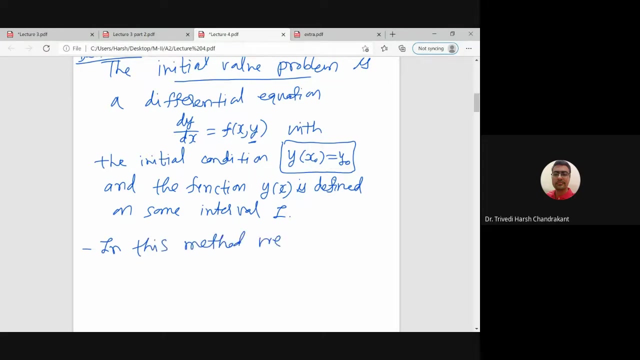 should be continuous function right, because basically what we want is we know that every from the mathematics one multivariable calculus, that every continuous function defined on close interval is bounded right. so in this method we shall usually consider the continuous function, the function F, to be continuous. 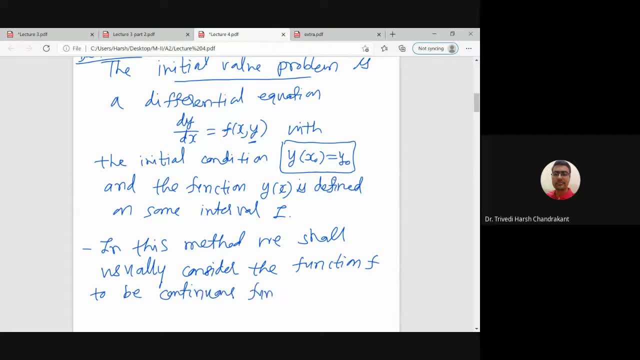 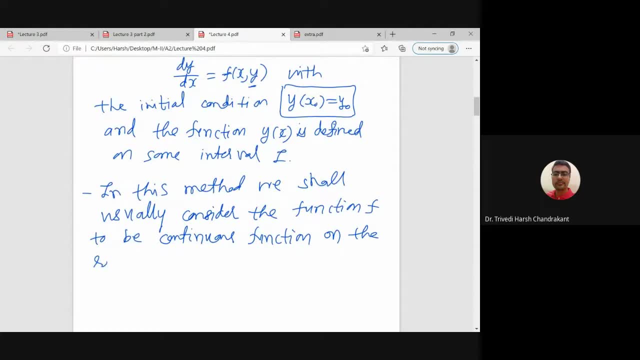 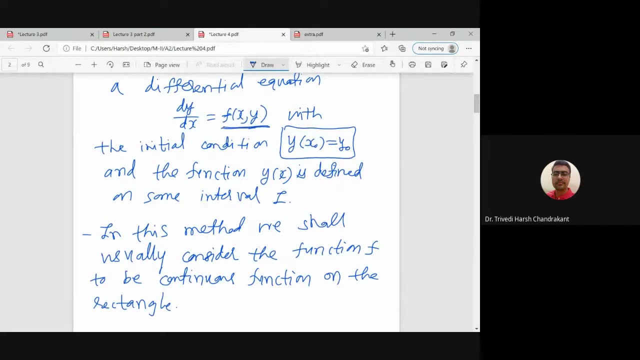 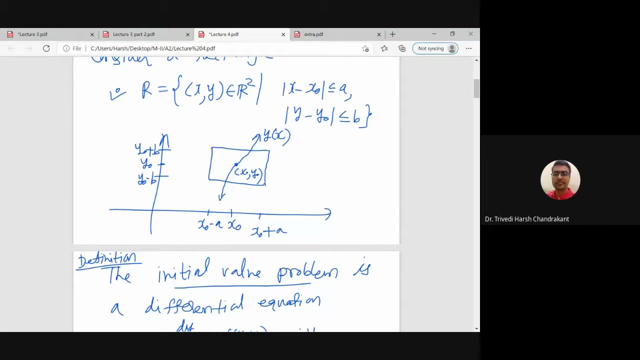 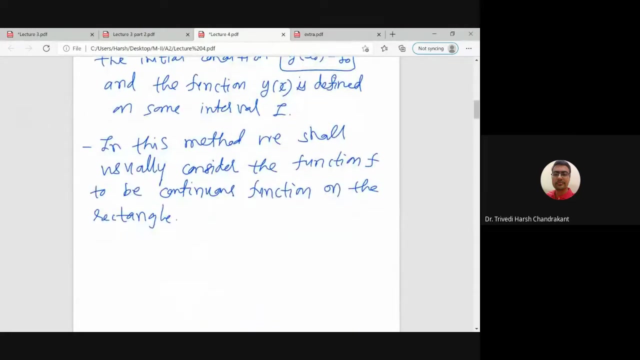 function on the domain. so domain is here is the rectangle. so you can see that F is a two variable function. F is a function of X and Y, right? so therefore we can define it over this whole rectangle, rectangle R. so usually we assume that the function is continuous over the rectangle R. so 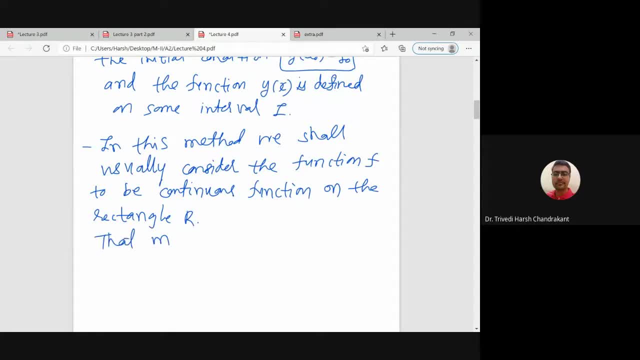 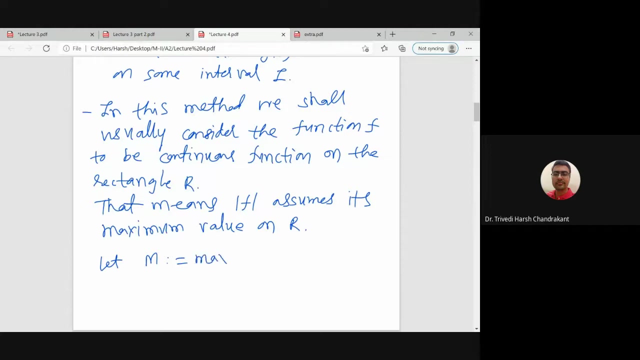 that means what that means? it assumes it's the, its modulus. so F is continuous. then modulus of is also continuous, so modulus F assumes its maximum value over the rectangular. so let's Let us call this maximum value to be m. So what is m? m is the maximum value of modulus of fxy, where this point xy belongs to the rectangle. 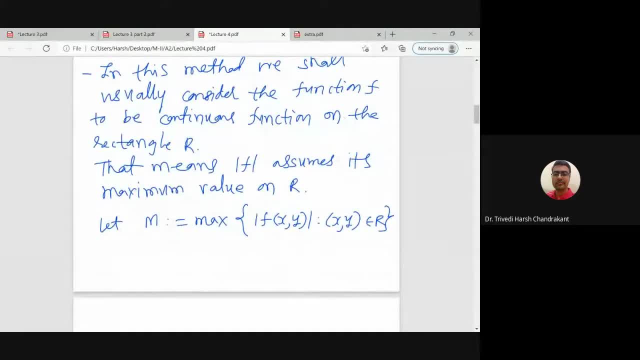 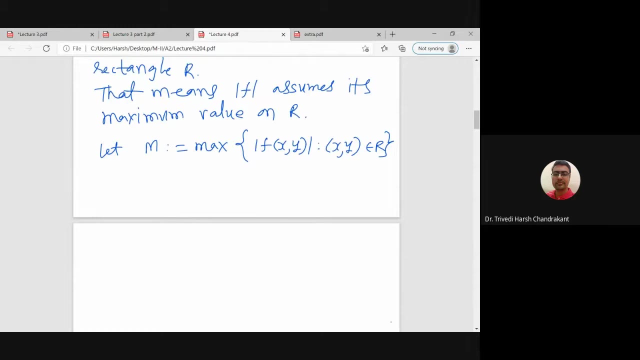 Right. So m is the maximum value of mod f function, And such a problem is called the initial value problem. So now let us see some examples of the initial value problem first. So we want to Yeah, any question? 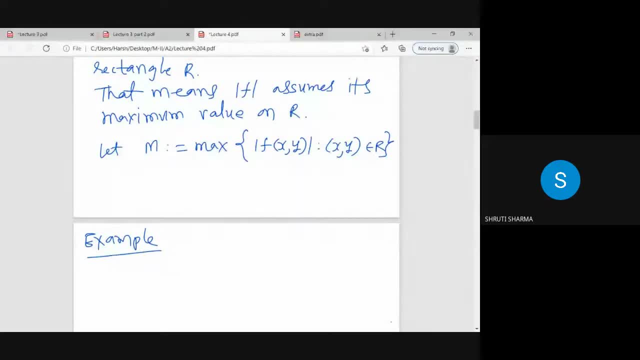 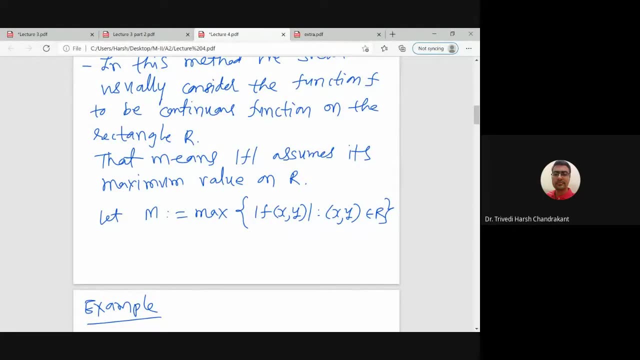 So how mod f assumes its maximum value on R. So we know that if it is a single variable function and the function is defined on the closed interval a- b, then it always assumes its maximum value. Continuous function over the closed interval always assumes its maximum value. 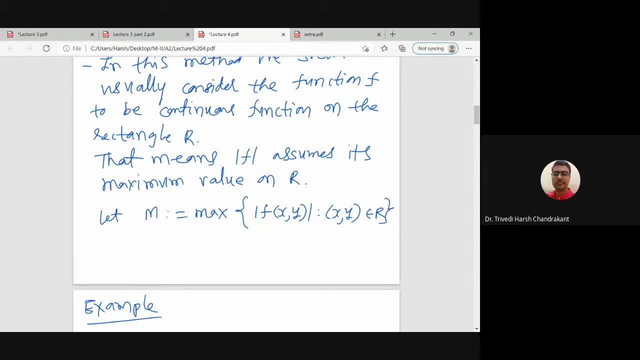 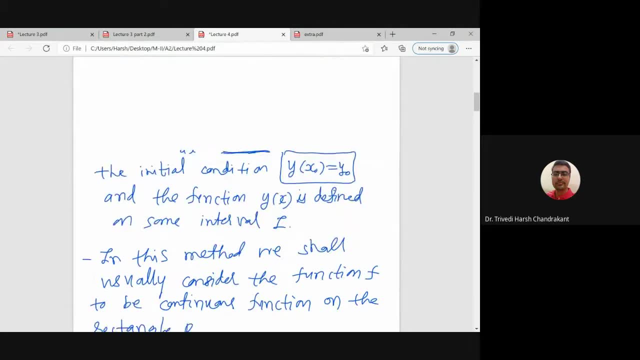 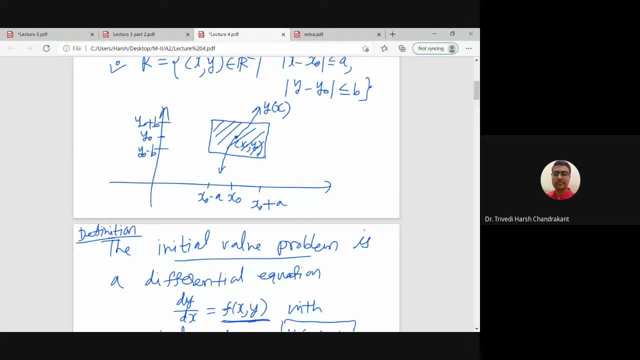 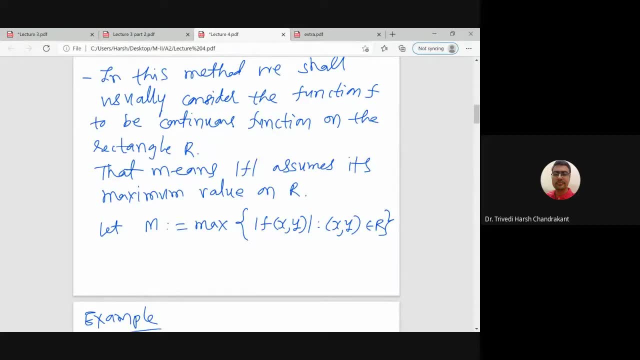 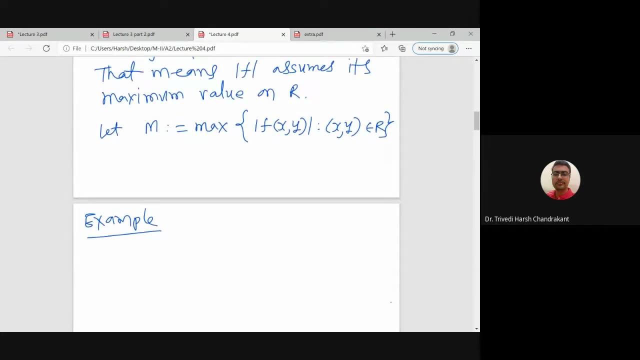 So here our set is a circular region, is a closed and bounded set which contains all its boundary points, so therefore it assumes its maximum value. and whenever f is continuous, modulus, f is also continuous, so that also we have discussed. so both of these things we are using here. 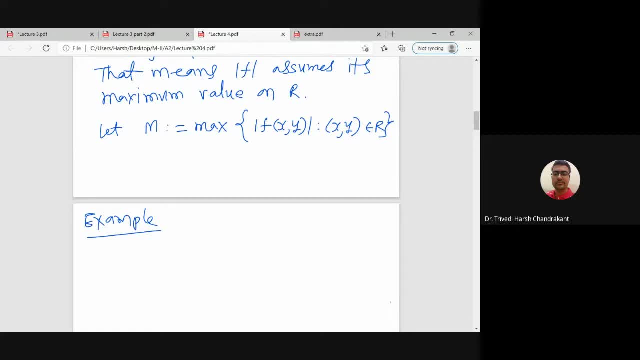 so you can try it by taking some example of two variable function and you can take a rectangle and you can try to find the maximum value right. so one of the method. also we discussed lagrange multiplier method, how to find maximum value of the function over the closed regions. 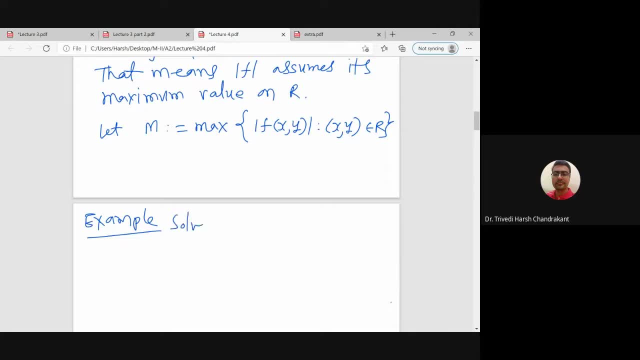 okay, so let me discuss one example of initial value problem. so we want to solve this differential equation. x y dash is equals to y minus 1. where x y dash is equal to y minus 1, where initial condition is given to be y 0 is equals to 1. 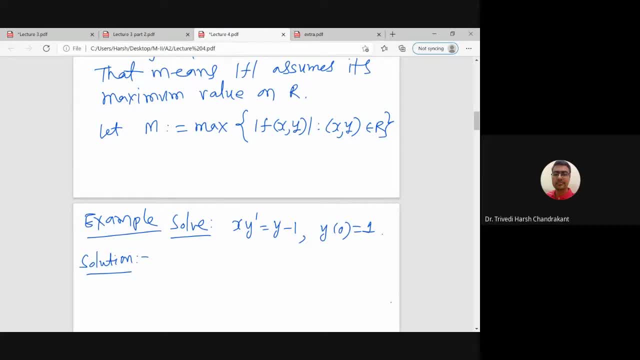 yeah. so this differential equation is a very, very simple differential equation. it is a separable, it is in the separable form, separable variable form. and the condition y x naught equals to y naught is y 0 is equals to 1. so that means basically here x naught is 0 and y naught is 1.. 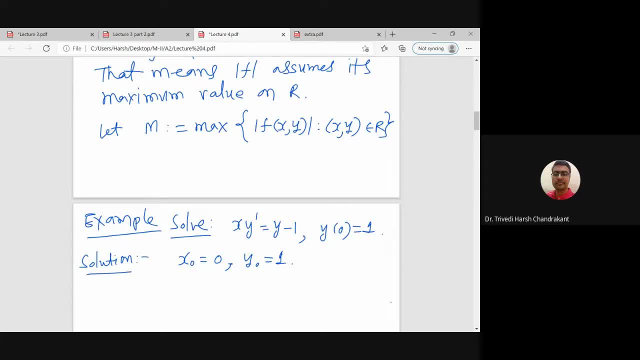 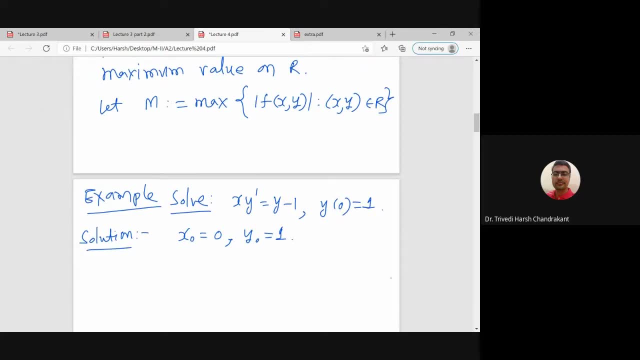 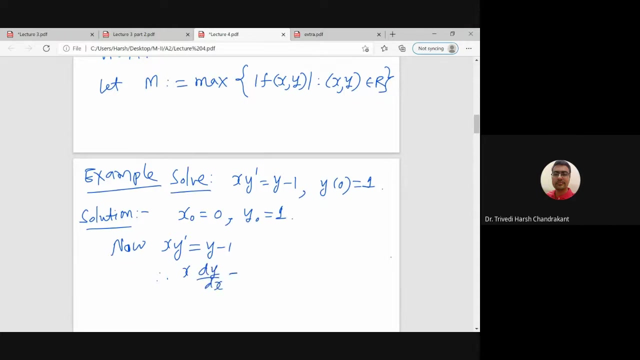 y naught is the value of the function y at the point x naught. so let us first solve this differential equation. so we have differential equation x. y dash equals to y minus 1. therefore x times dy by dx equals to y minus 1. gives dy by y minus 1 is equals to dx by x. 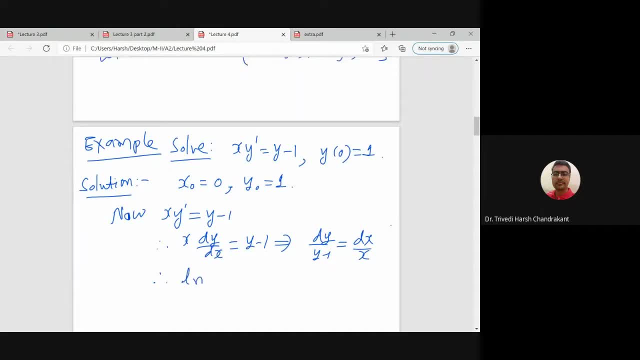 and integrating it, we get: logarithm of y minus 1 is equals to logarithm of x plus log c. right, and this will gives us so. in fact we need to consider here modulus. so essentially what we get is we can consider this to be log more c, so it will be y minus 1. 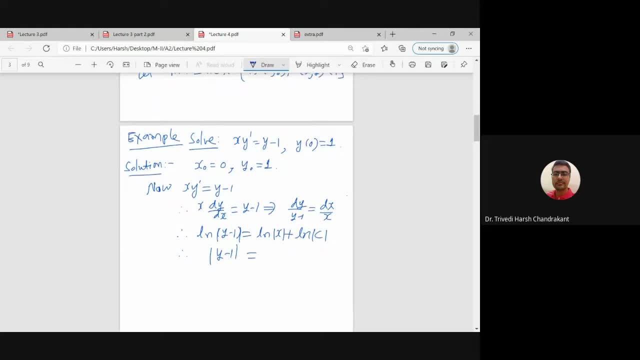 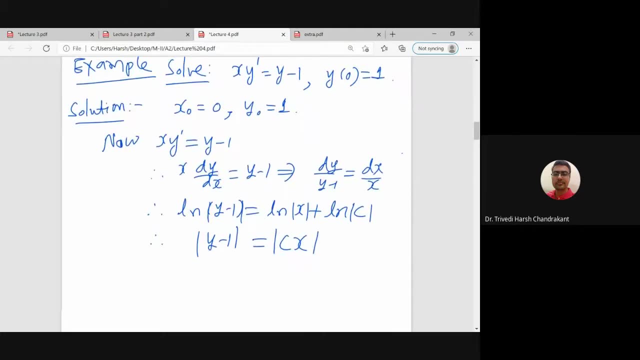 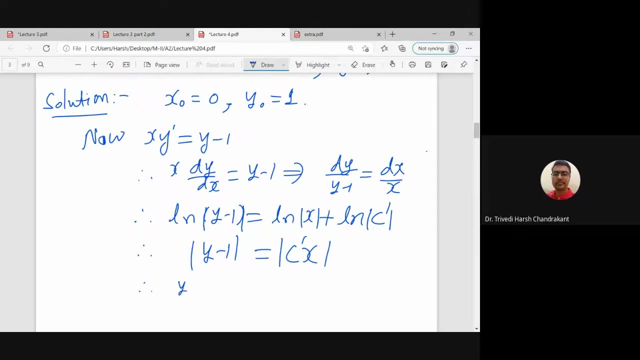 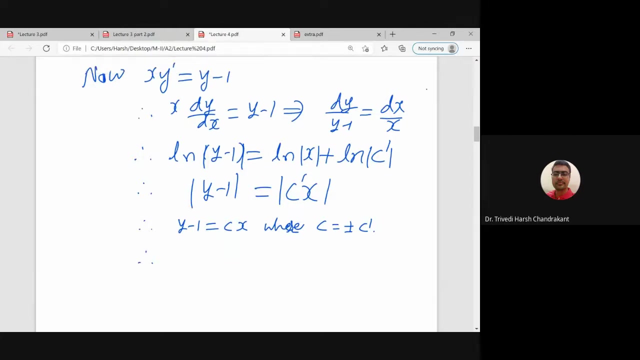 modulus is equals to modulus of cx, right, and since C is a constant, we can even rewrite, we can call it C dash and finally, anyway, we will get this: y minus 1 is equals to C times X. where C is, we can say plus or minus C dash, right. so basically we can, we want to. 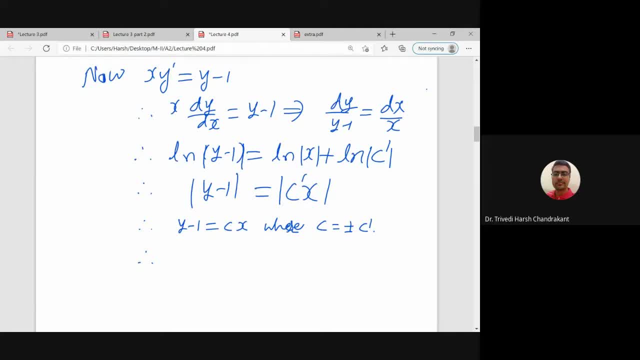 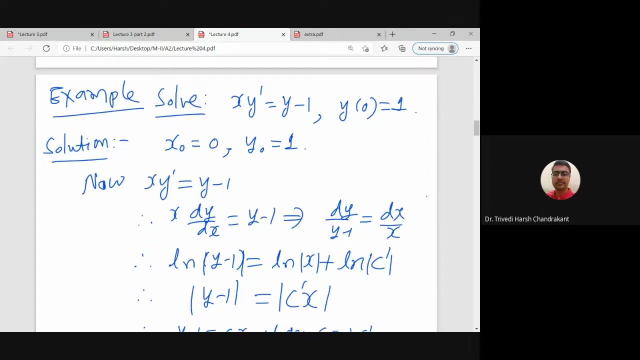 remove the modulus. so that's why we change the constant from C dash to C and finally we get the solution to be C X plus 1, where C is some constant. so, given differential equation, because it was of the separable variable form, we have solved it and we got the general solution. but what is our question? we 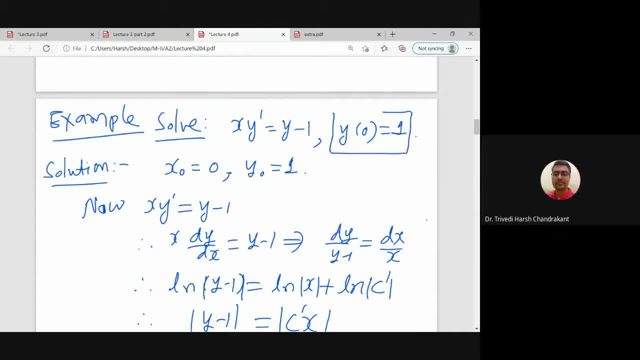 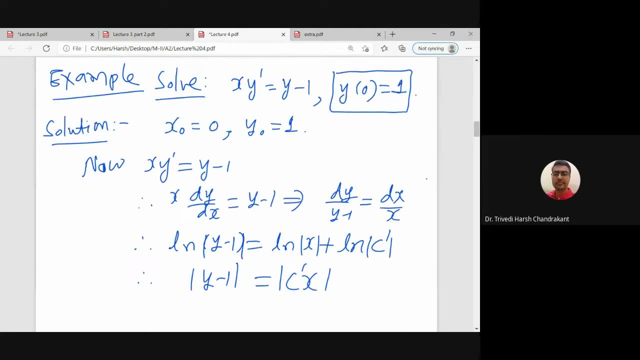 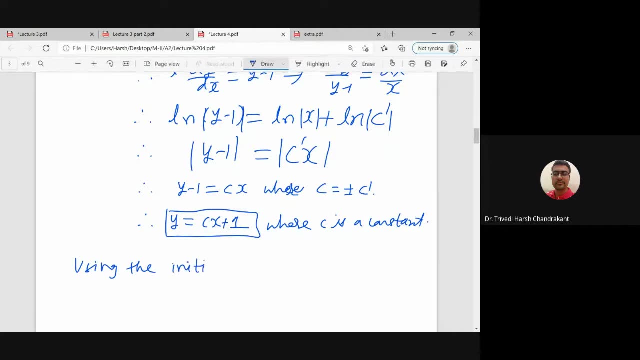 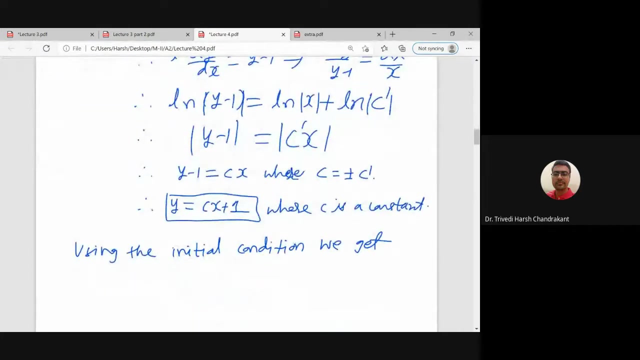 want solution Y, which satisfies the initial condition, so that means it passes through the point 0 comma 1, right? so if we substitute here using the initial condition, what we get is: whenever we substitute, initial condition is y, 0 equals to 1, so that means, whenever we substitute the value 0 in 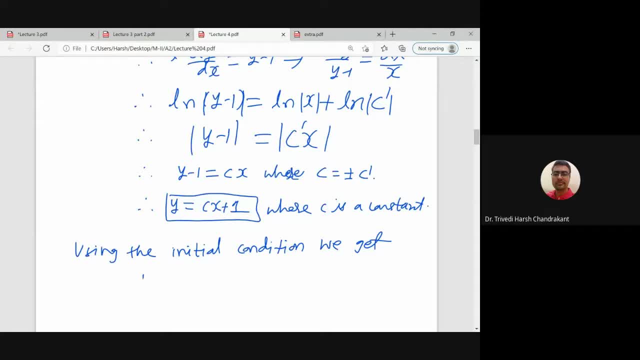 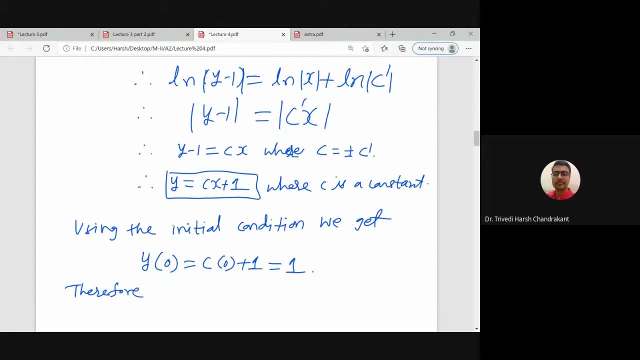 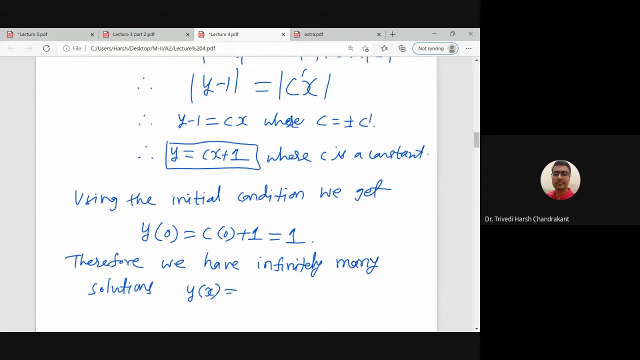 this function. so this is y X. so what is y 0? y 0 is C times 0 plus 1, so that is always 1 right. so therefore we have infinitely many solutions which can be given by y X equals to C X plus 1 of this. 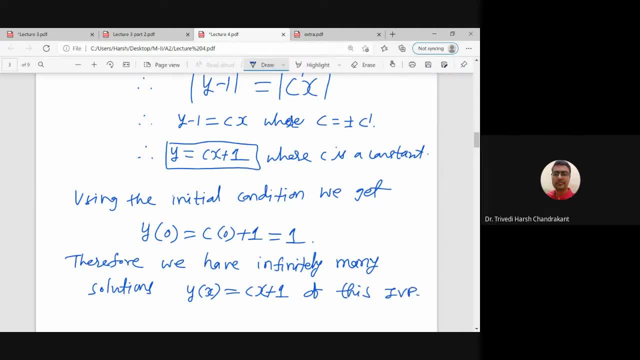 initial value problem. so usually we write IVP in short. so why there are infinitely many solutions? because we can choose different values of the constant C. we can take: C is equals to 1, C equals to 2, C equals to minus 1, right. so depending on that, we get infinitely many cows, y, X, which satisfies this. 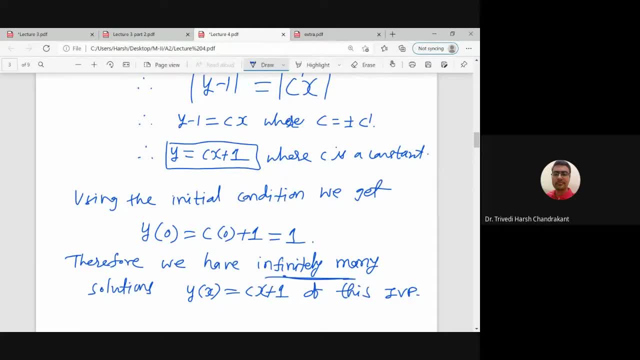 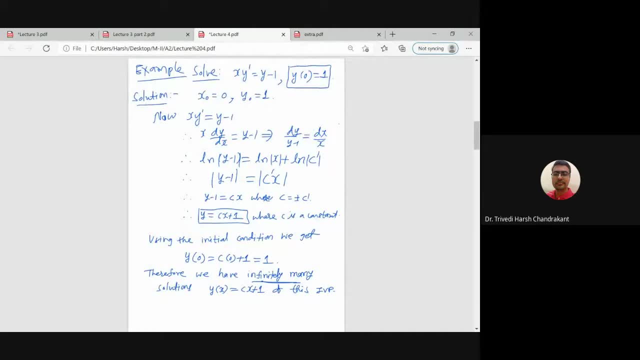 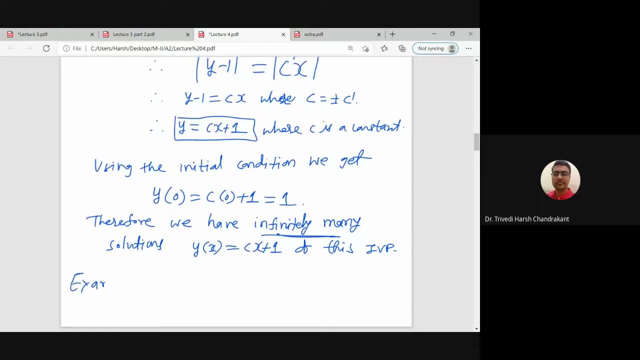 differential equation. so these first example of the differential equation is the of initial value problem, where we are getting infinitely many solutions. let us see the another example. so if I consider the same differential equation, solve X, Y dash is equals to y minus 1, where y of 0 is equals to 2. so then how many? 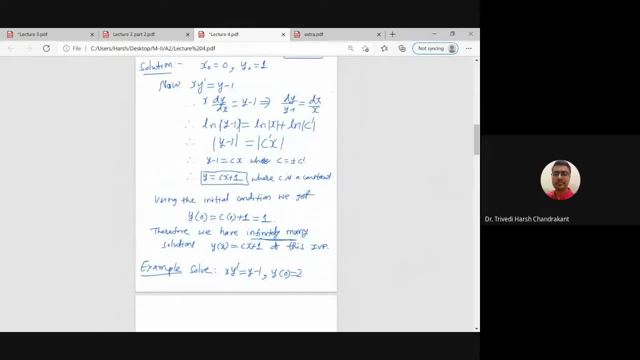 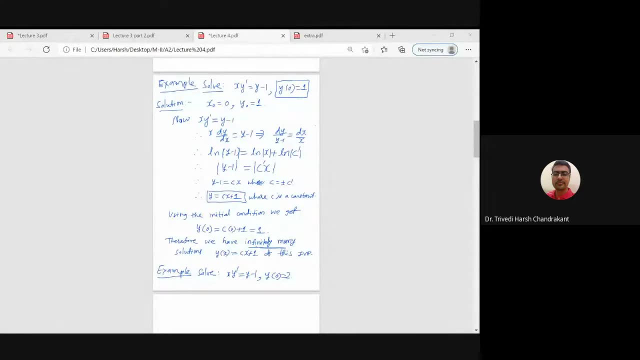 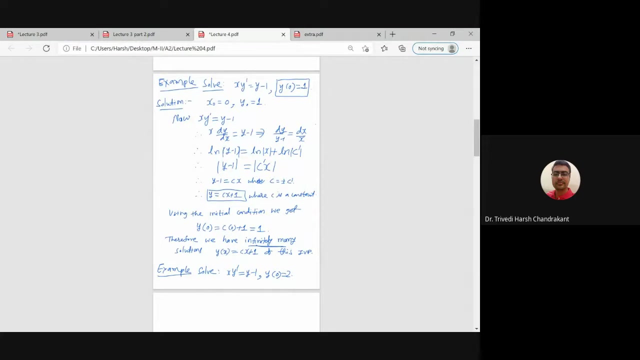 solutions this differential equation has. so we are taking differential equation, same, but the condition be changed by y 0 equals to 1, 2, y 0 equals to 2. no solution, no solution, right, because all these cows satisfies: y 0 is equals to 1, right? so this differential, this? 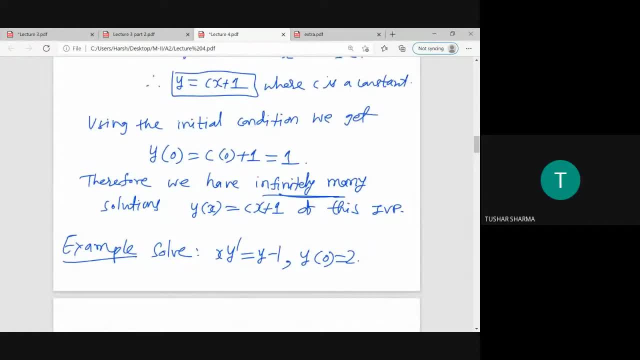 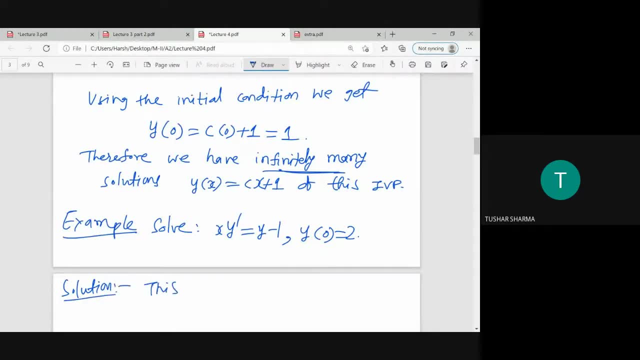 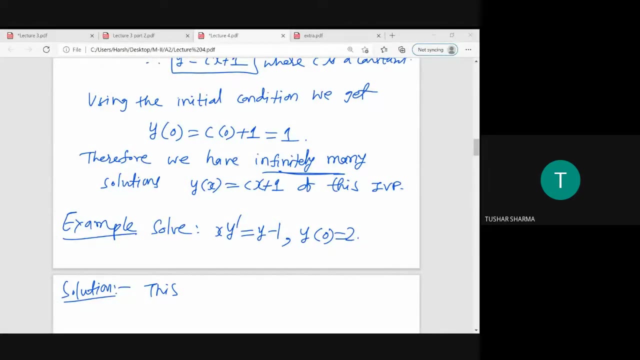 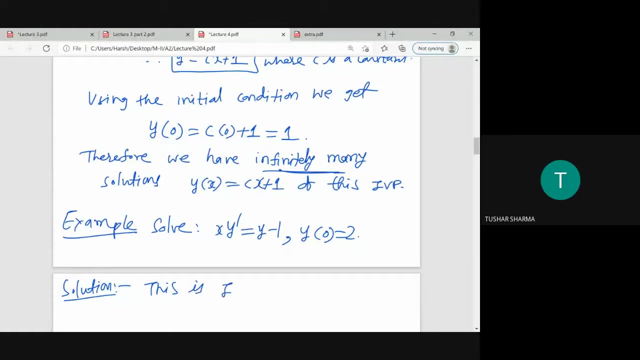 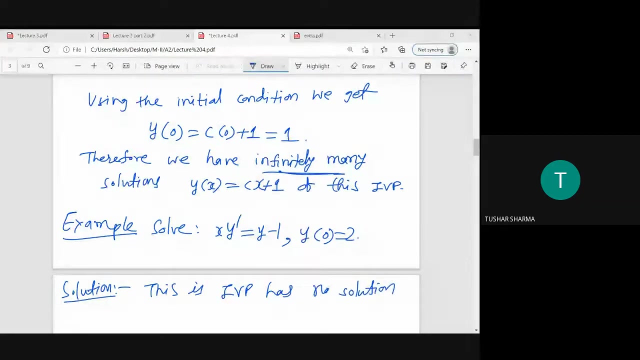 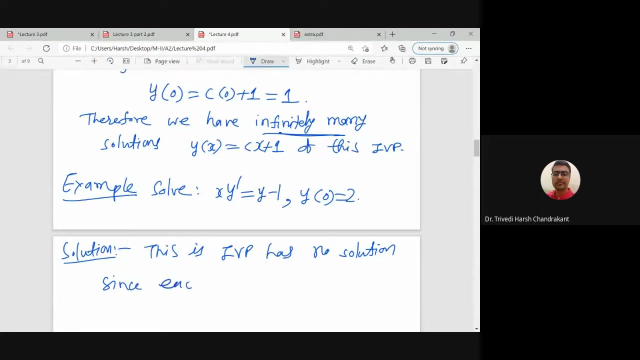 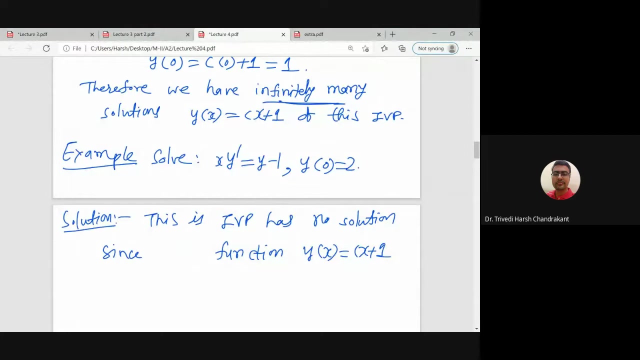 initial value problem has no solution. yes, any question. so this initial value problem has no solution, you, you, you. since each go y, x is equals to cx plus 1 local, no function satisfy you, you. the condition y 0 is equal to 2, so this initial value problem has no solution. so 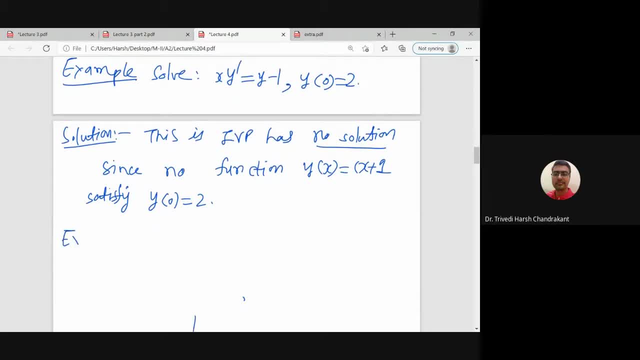 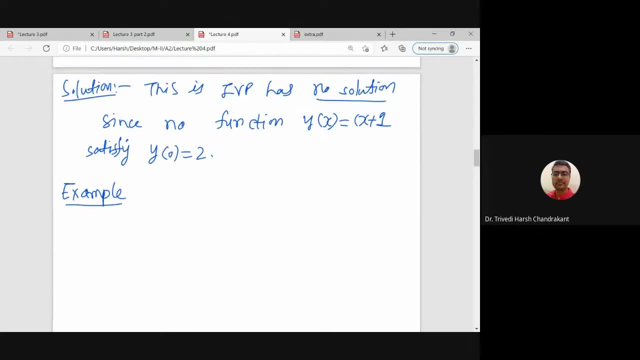 previous example as infinite solution. this has no solution. so what about the unique solution case? so let us see one example of the unique solution. so we want to solve the differential equation: y dash is equal to 2x, where y 0 is equals to 1. 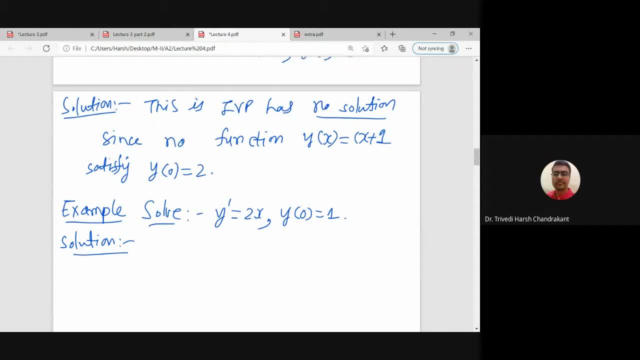 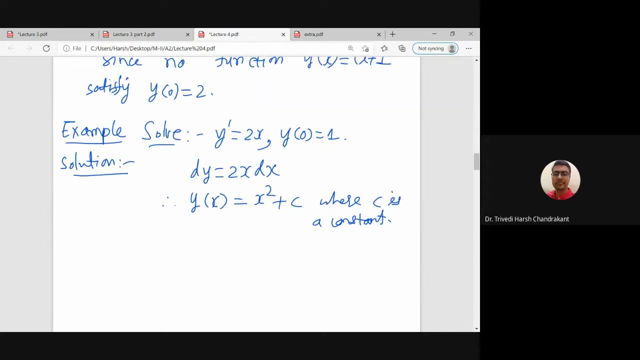 so here also, this differential equation is a very simple differential equation. we can separate it and we get the solution: y x equals 2. if we integrate it, we get x square plus 1. this is constant and using, if you use the initial condition, we get: y 0 is equals to 0 square plus C is equals to 1. right, because y 0 is 1. 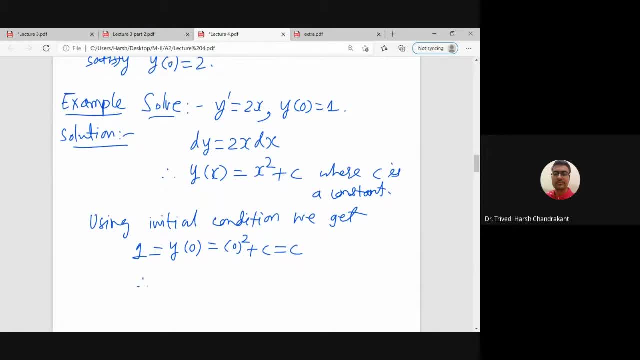 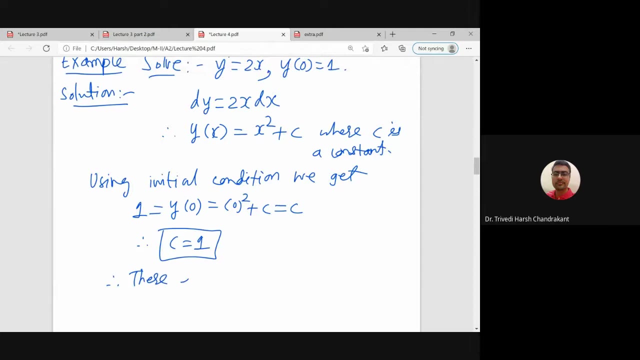 so this is c, so that will give us the value: of C is 1. then, and only then, the initial value, initial condition is satisfied. so that means there is only one solution for the constant value: 1, why x equals to x square plus 1 of this initial value problem. 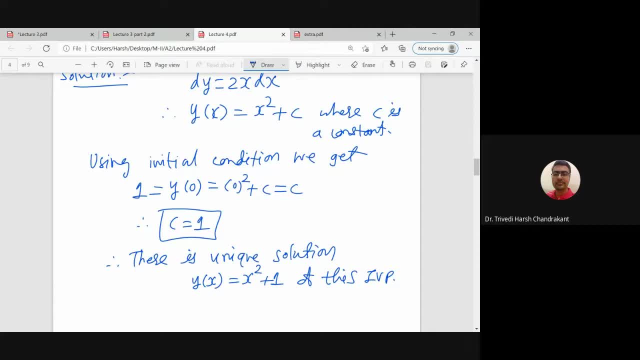 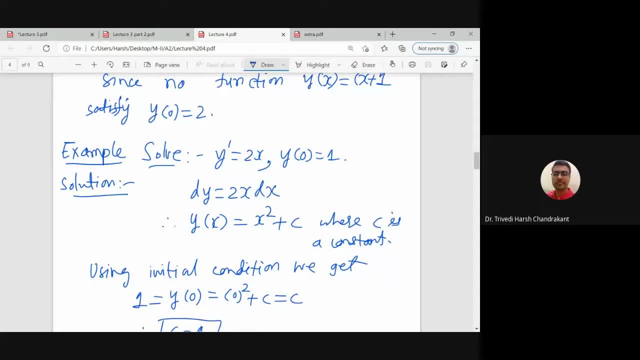 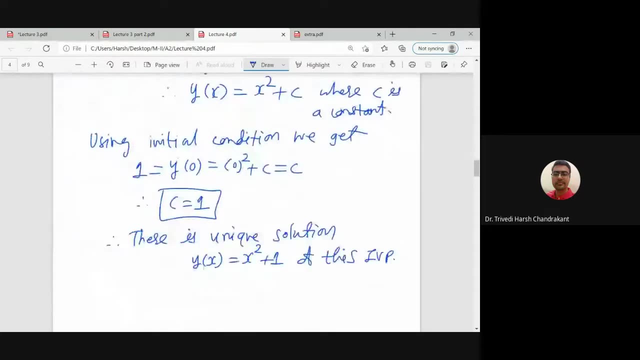 all right. so in these three examples we are taking the condition in terms of zero, y zero, but we can also take evaluate y at different other points also, depending on what is x naught given. the only thing is to mention here is that the initial value problem may have different type of solutions. 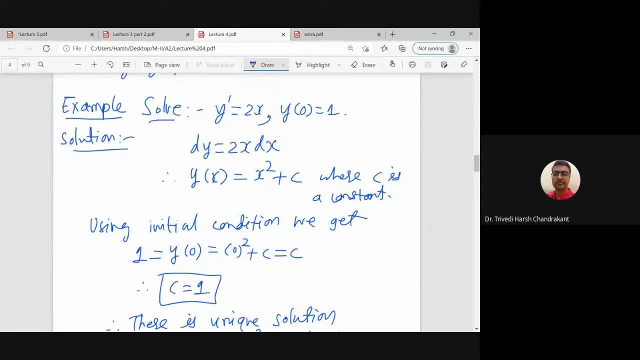 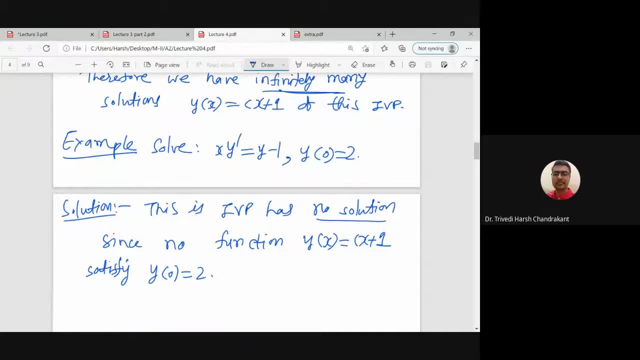 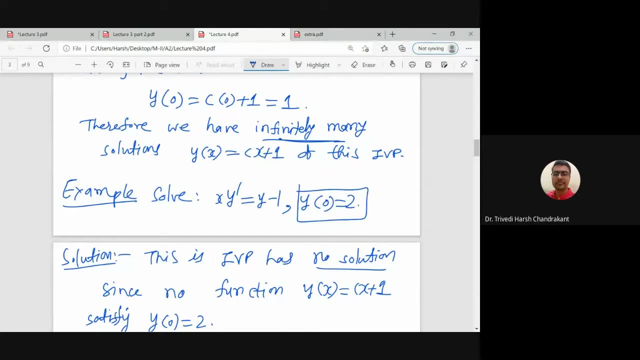 and in. in these cases we can see that that it has unique solution, no solution or infinitely many solution. that depends on the value of c and this initial condition. right, so, that way you can relate, uh, these two concepts. so now let us move to the method: how to solve. 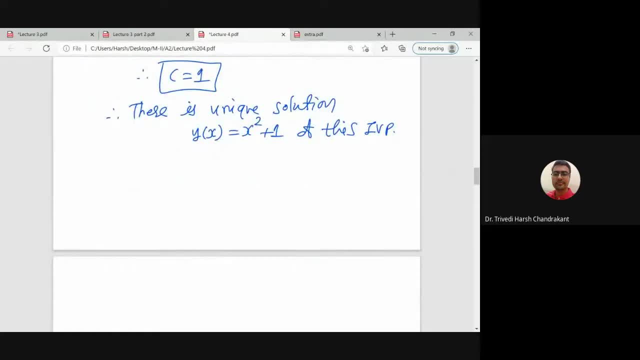 initial value problem if the solution exists, or in other words, how to find the solution using the approximation. so this method is known as picard's iteration method, so picard's solution method to find a solution of initial value problem. so let us see this method. so basically, we want to solve: 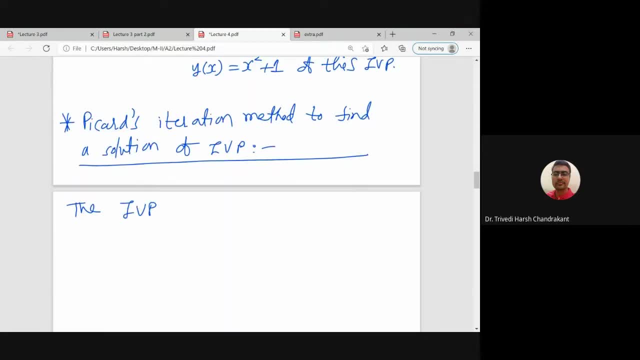 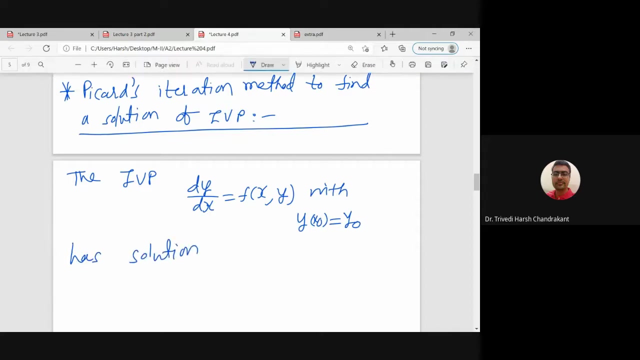 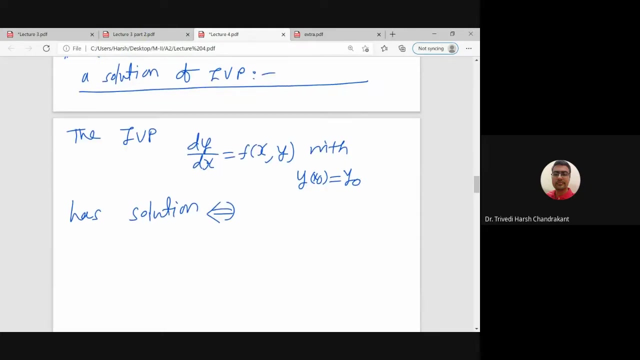 the initial value. problem dy by dx times y into x is equal to f of x. y. with the initial condition y of x, not is equals to y. naught has solution if, and only if, we know that we can rewrite this same equation in this form: so yx equals to y. 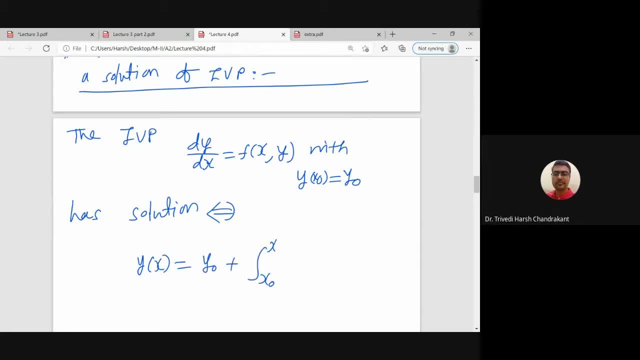 naught plus integration, X naught to X, f of t, yt, dt. so if we saw, if we differentiate this equation, we studied the fundamental theorem calculus. so what is this? X and Y? Y is basically the function of X. so that means this whole function we can consider as a single variable function, function of X. 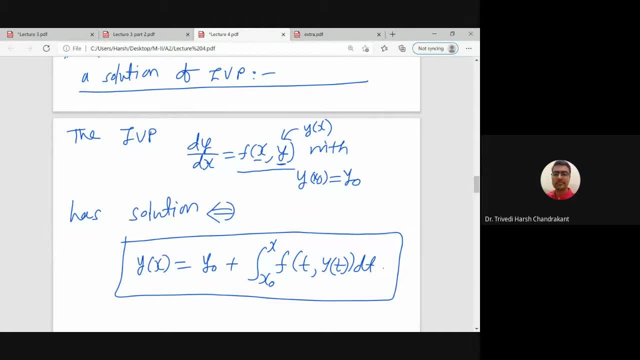 and that is, if we differentiate this part. what we get is we get f of X, Y, X. differentiation of y naught is 0 and derivative of Y is divided by dx right. so that means this integral equation is given. then we get the differential equation and on the other hand, if we integrate this differential 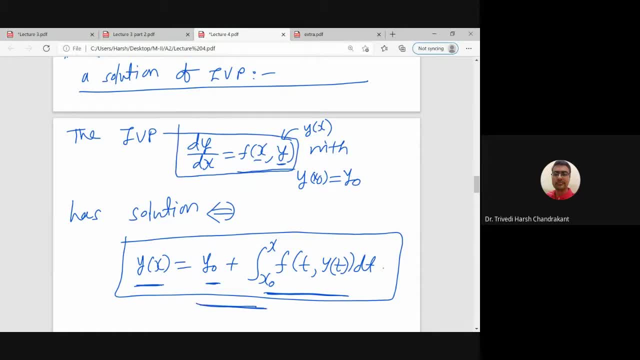 equation. we get this equation and then, using initial condition, we get the constant of the integration to be Y, naught right. usually when we integrate, we take the constant C, but that C turns out to be Y naught, using this initial condition. so therefore, this initial value problem has a solution if, and only if, 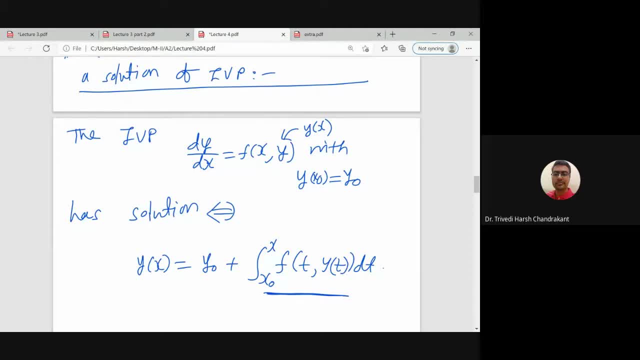 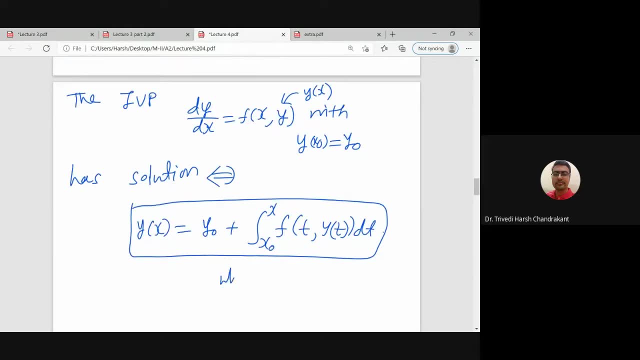 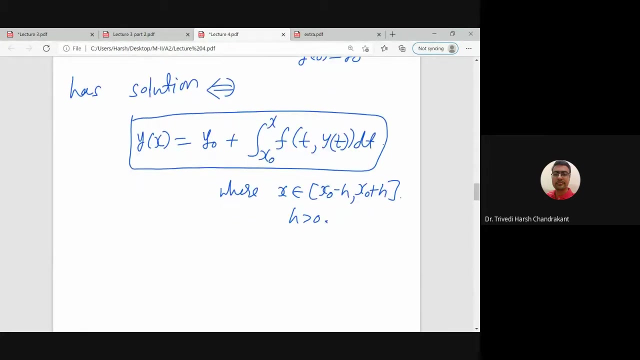 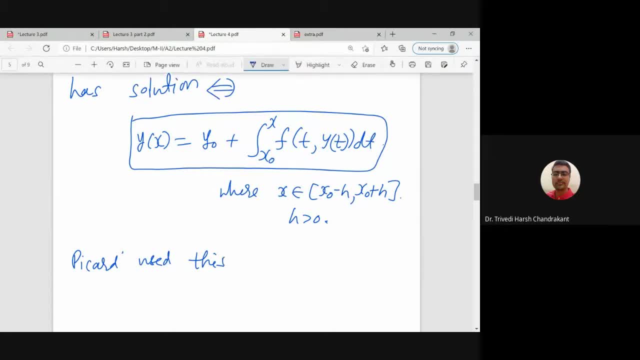 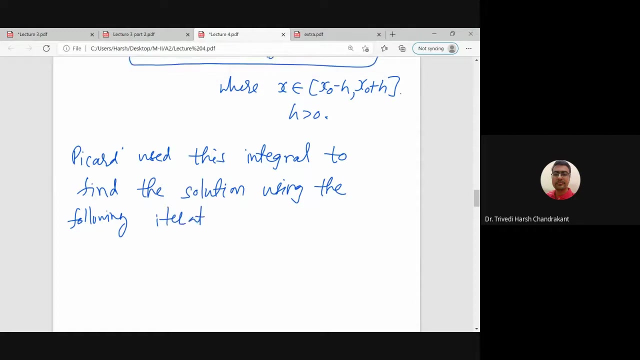 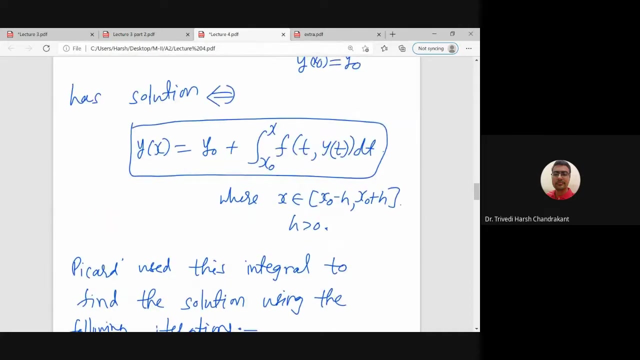 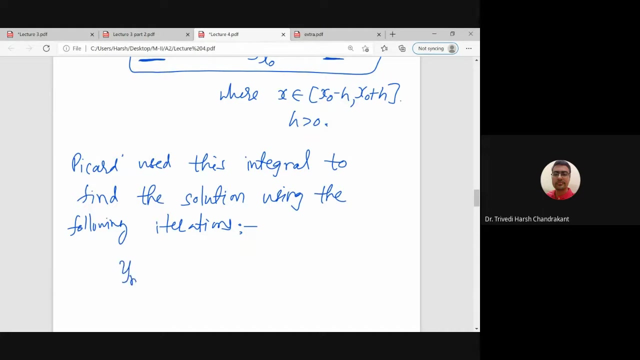 this integral to find the solution using the following iterations: so these iterations are known as quarts iterations. so what we will do first is we will substitute different functions here and on the other hand we will get these functions right. so they are the iterations. so the formula of this iteration is that the nth iteration, nth iterated function y is: 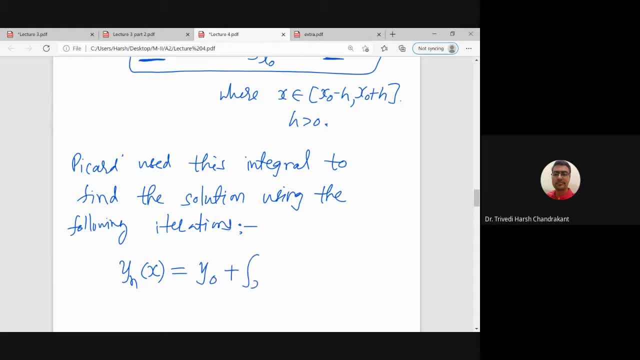 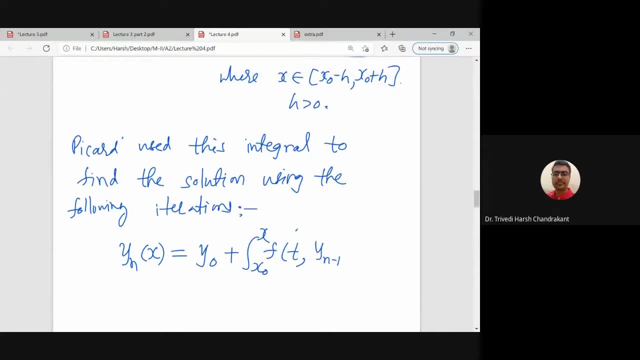 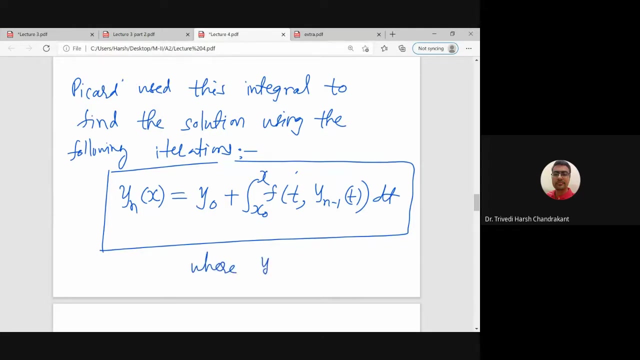 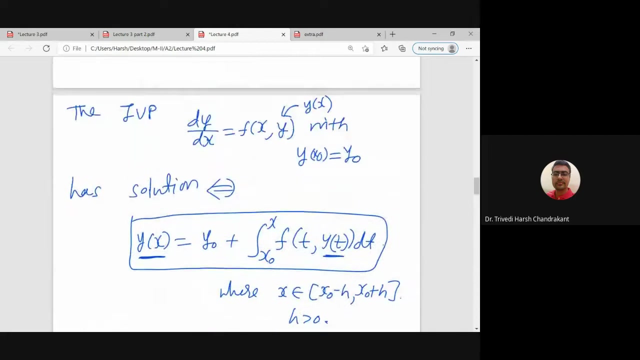 we can find using this integral formula by substituting n minus 1th iteration, right. so these iterations are known as piquart's iteration and where the first function which we will consider will consider to be the constant function, y naught. so what is y naught? y naught is the initial value, is coming from the initial value. 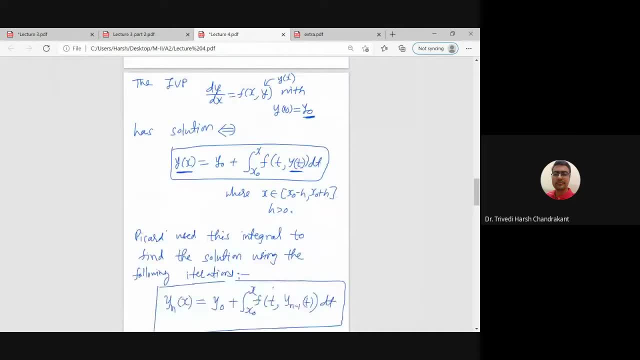 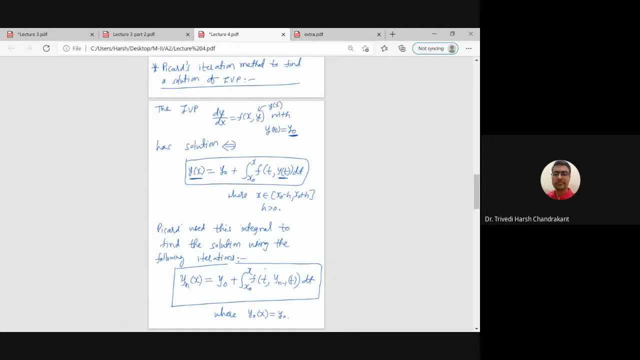 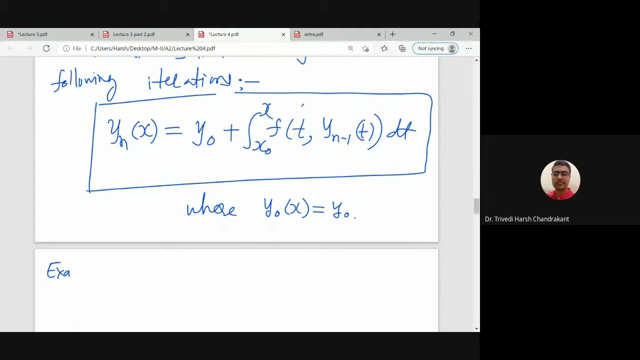 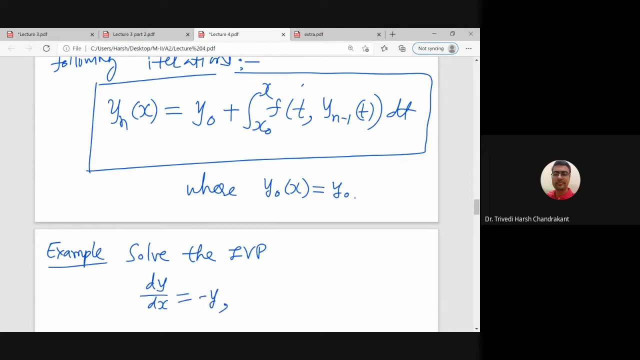 so by substituting y naught, we'll get y1. by substituting y1 in this iteration formula we get y2, and so on. so let us see how this method works by an example. by initial value problem dy by dx is equal to minus y. when the initial condition is given to be y0 is equal to, Y0 is equal to minus 1 and the value of X is between minus 1. 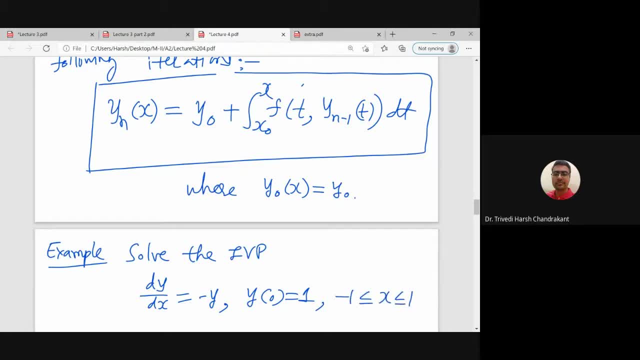 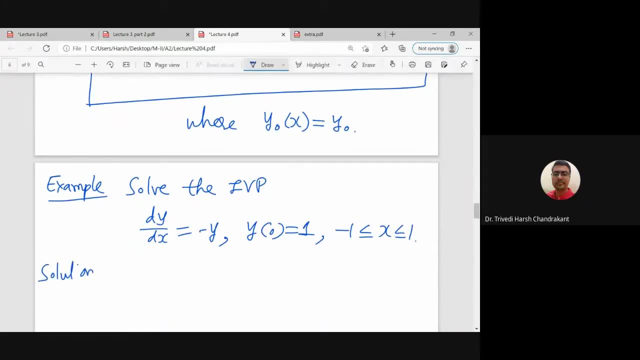 and the value of X is between minus 1 and the value of X is between minus 1 and one. yeah, so again, this is also a simple differential equation. we can use separable variable form and easily we can find its solution. but for instance, we want to apply the Picard's method. whether it works and can we find the? 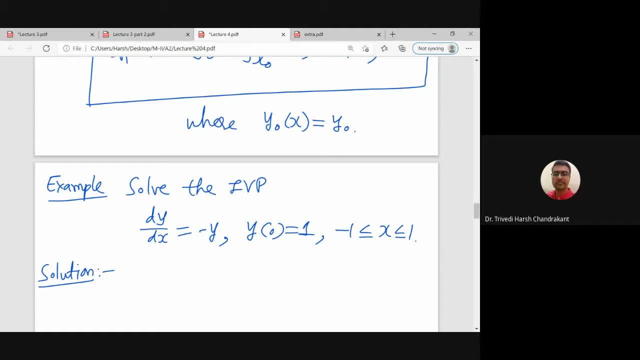 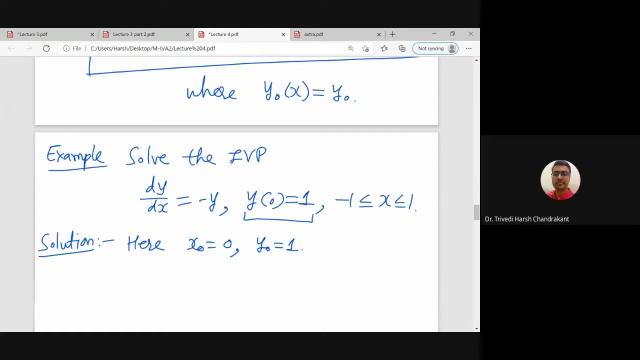 solution using the iteration methods. so let us see how this iteration method works. so note that here our X naught is 0, our Y naught is 1. right, because Y, X naught is Y naught, and so therefore, the first function we will consider is Y. 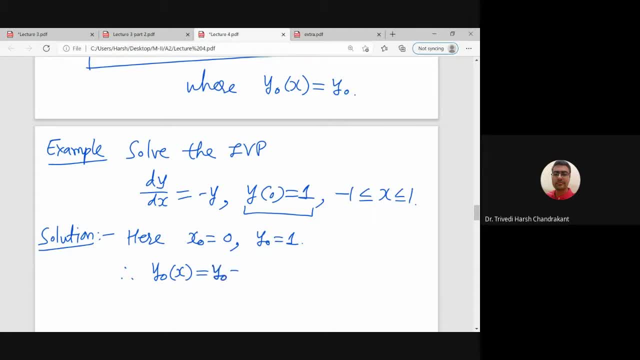 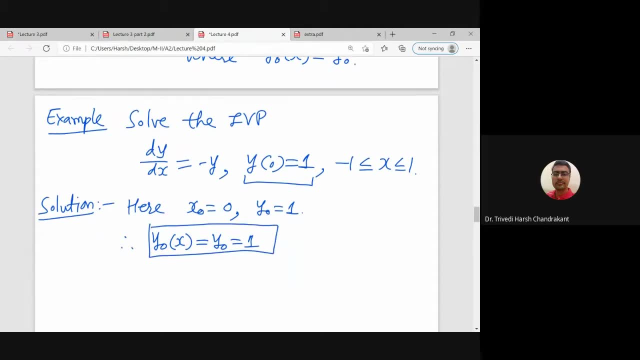 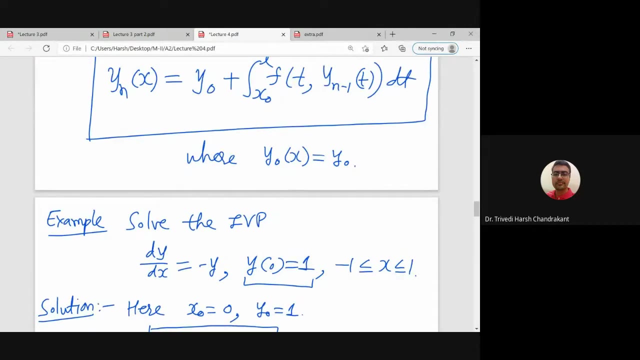 naught X to be the Y naught function, and that is constant function 1. so using this first function, Y naught, let us apply the Picard's iteration formula. so for n is equals to one, we get y. 1 of X equals to Y naught. and here we 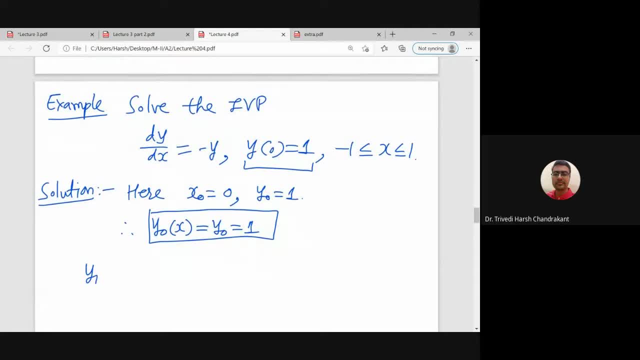 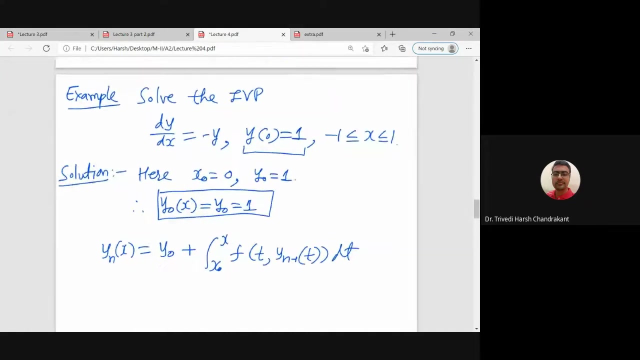 suffice with Y zero. So y 1 of X is equals to Y naught. Ya. so let us first write down the general formula. so Yn of X equals to Y knot is 0.. is equals to Y, naught is 0.. plus x naught to x. f of t, y naught t, sorry, yn minus 1 t dt. so this will give us, we know, y naught. 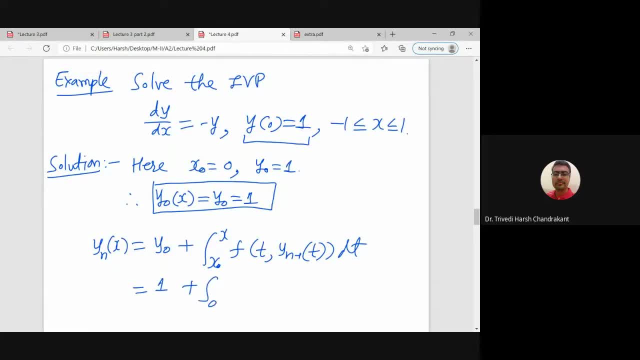 is 1 plus integral x. naught is 0 to x, f of yeah. so what is the function f here? the function f is minus 1, so these two are given and the function f, x, y is given to be minus 1, right, whatever is. 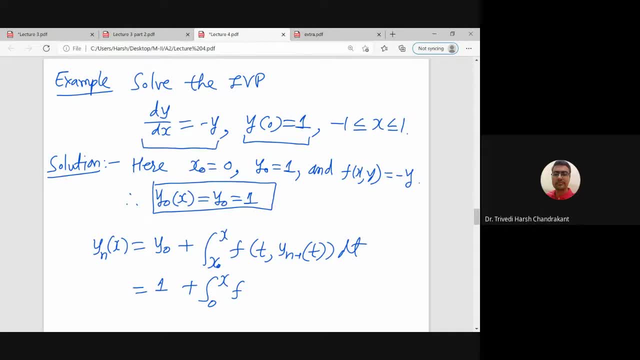 on the right hand side of this equation, divide by dx equals to 0, something, that something is the function f. so now, if we substitute that function f here, that means we need to integrate the second part, y part. so that is yn minus 1, t, dt, right, so this is the. 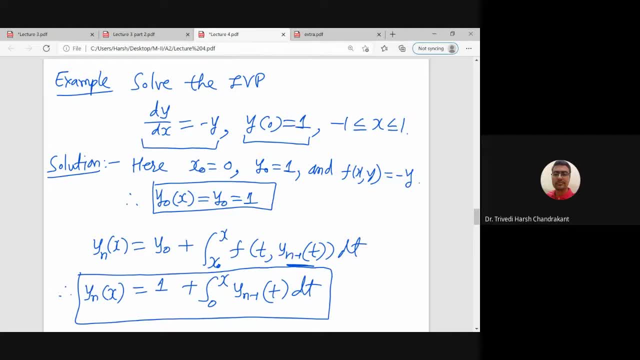 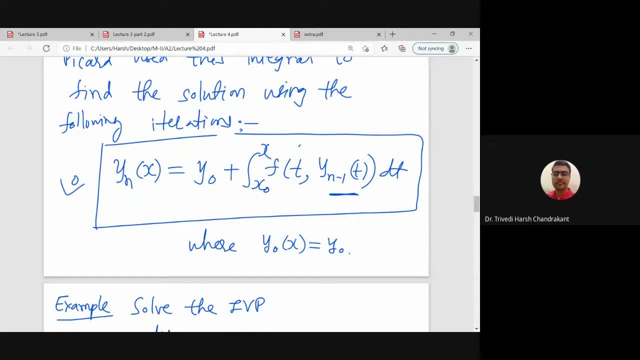 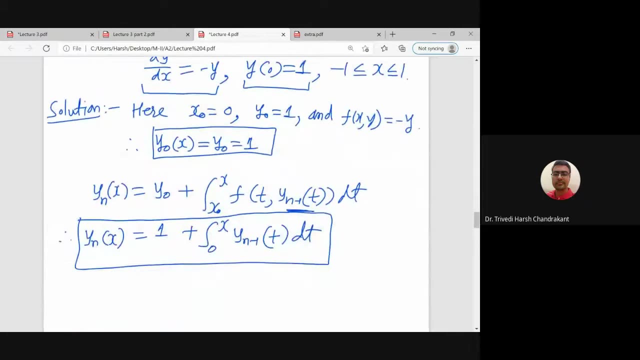 picard's iteration for this particular example. so in general, picard iteration formula is this one, but whenever we substitute the initial condition x naught, y naught and the function f, we get the picard's sẽ tentation formula for the given example. that is this one. and then we step by step, one by one, substitute. 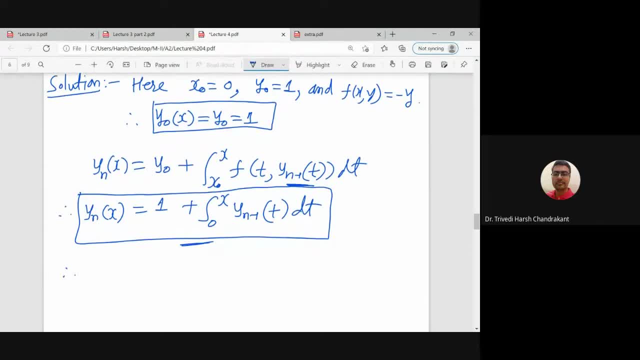 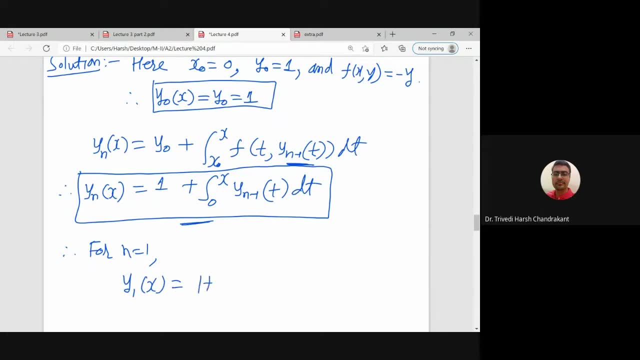 the iterations. so now for n equals to 1, this formula gives first iteration, that is 1, plus integral 0 to x, y, 0. so y, 0 is the initial condition. i" that is one, will express the teacher's expression below, and the formula 0 is expressed沒有. so means 0 is the first. 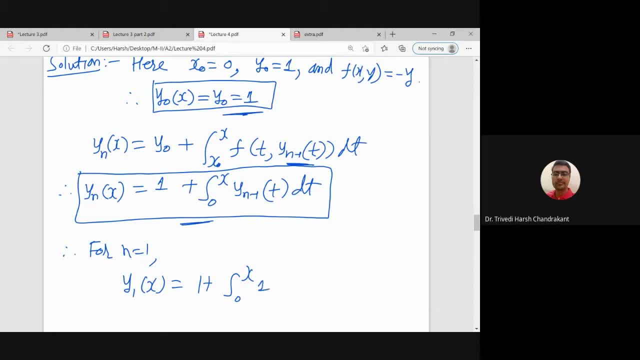 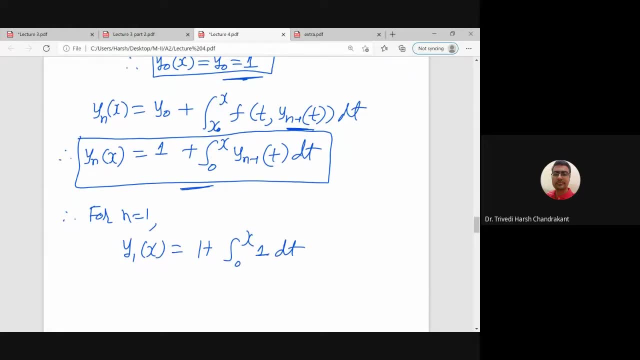 day of integration. n equals to one to x. ok, from the that we can add one minute of 1080. that's 1. for this, 0 is 1, that is 1 DT. so I think I did mistake. that should be minus 1, so that. 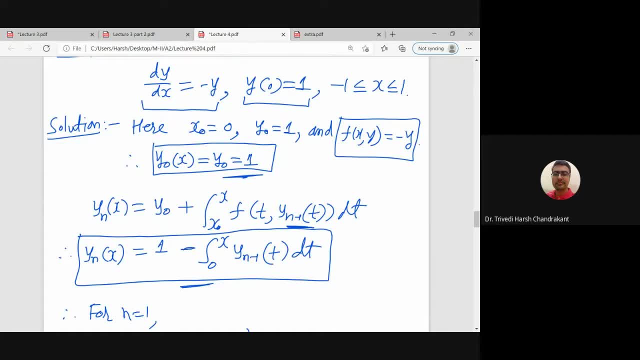 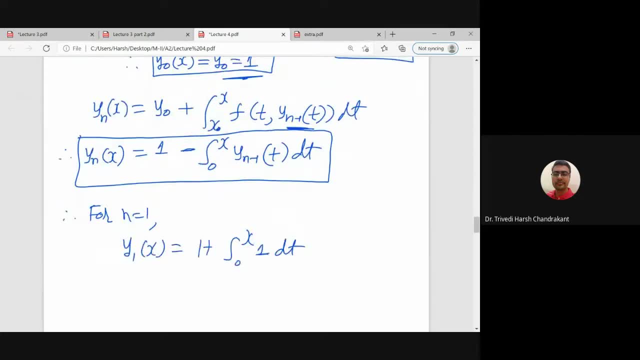 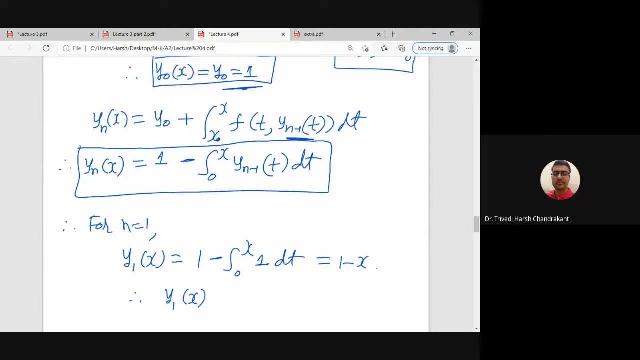 means the function F. I have substituted wrongly for X. Y is minus 1, so that means this is the general formula. it will give us minus value here and that will give us 1 minus X. so this is our first polynomial. first polynomial was Y, naught is 1. second polynomial is: Y1 is 1 minus X. 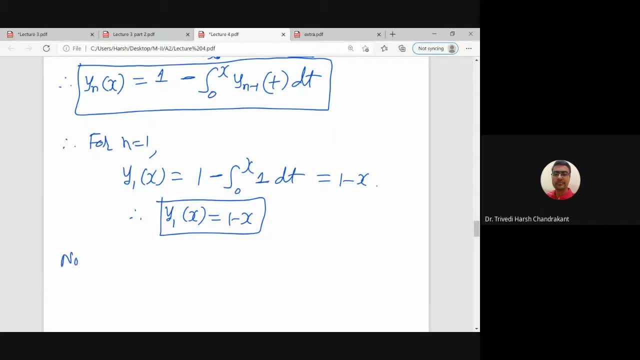 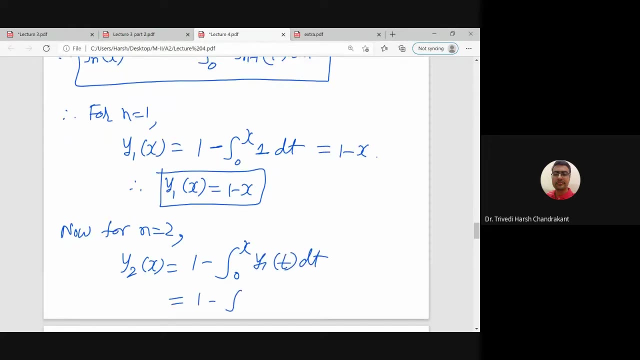 right. so now for n is equal to 2, we get Y2. X is equals to 1 minus integral 0 to X. Y1 T DT. so that is 1 minus 0 to X. Y1 T is 1 minus T in terms of T variable. right, this is x variable. 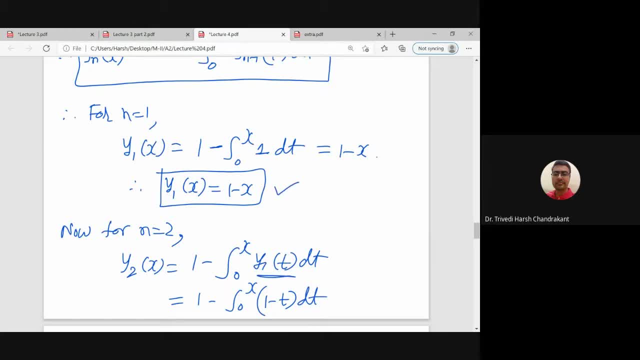 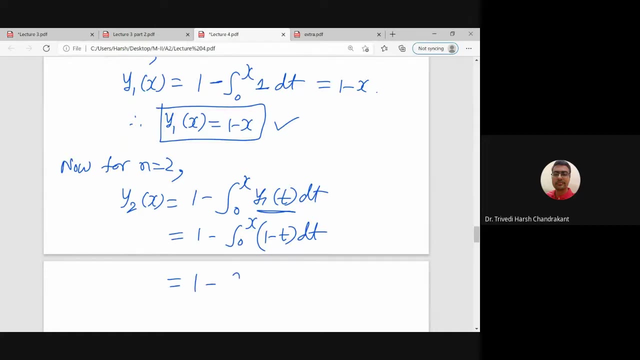 now we have to substitute in T variable, so we need to integrate 1 minus T, so that will gives us 1 minus integral. yeah, so this will be t minus t, square by 2, 0 to x, so that will gives us 1 minus t. 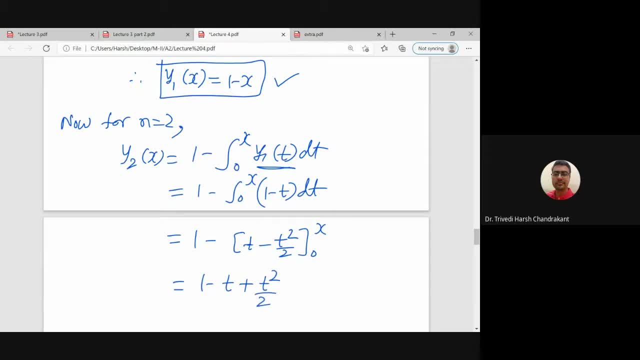 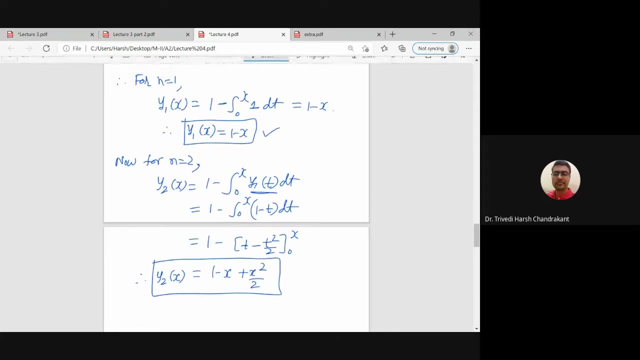 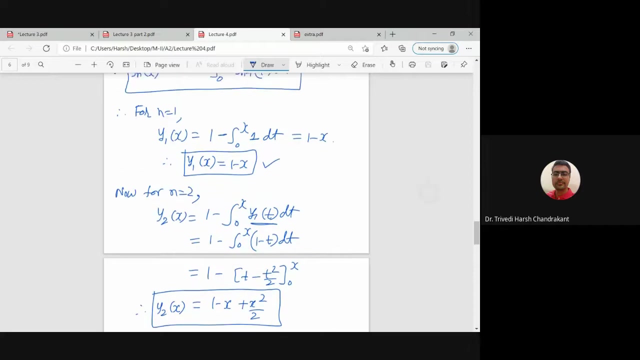 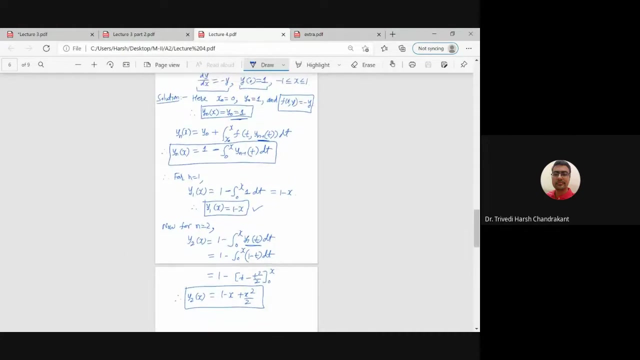 plus t square by 2. so that is our yeah. so we need to substitute x variable as t. that means it will be x square by 2 is our second polynomial. so now thing is that we need to guess the nth term of this polynomial. first term is y. naught is equals to 1. second term is second polynomial: y1 is 1. 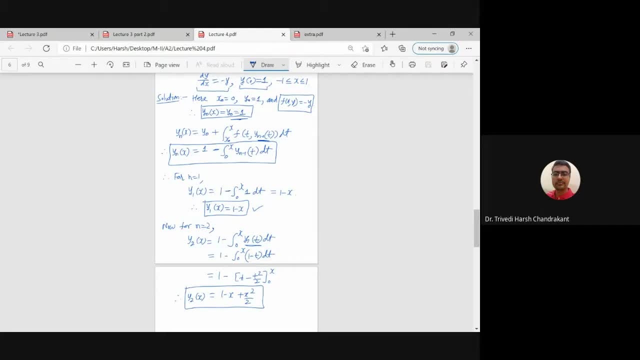 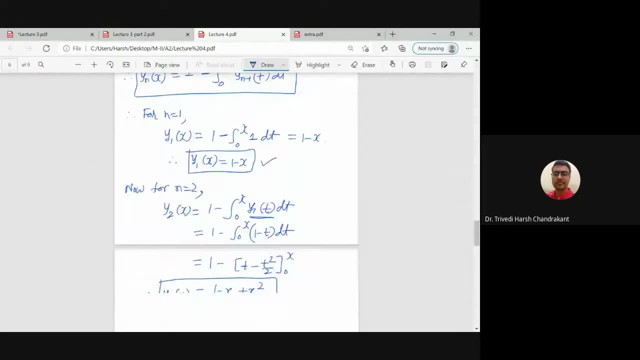 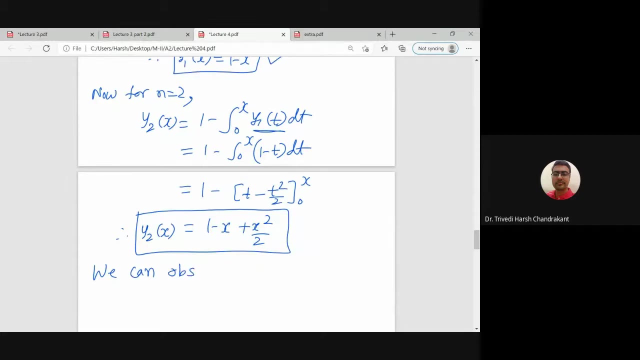 minus X. third column is: y2 is 1 minus X plus X square by 2. so this gives us a general idea that what should be the nth term. so we can observe that or verify that the nth term, nth function, ynx will be 1 minus X plus X square by 2, factorial. 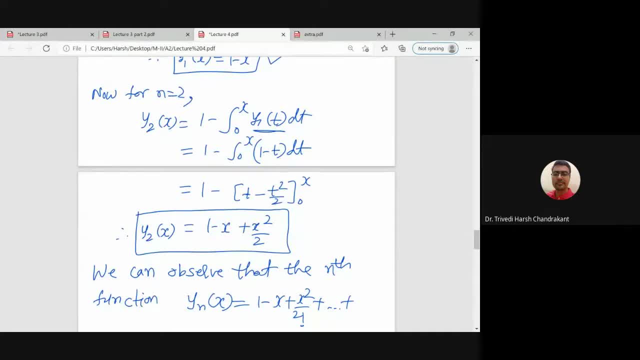 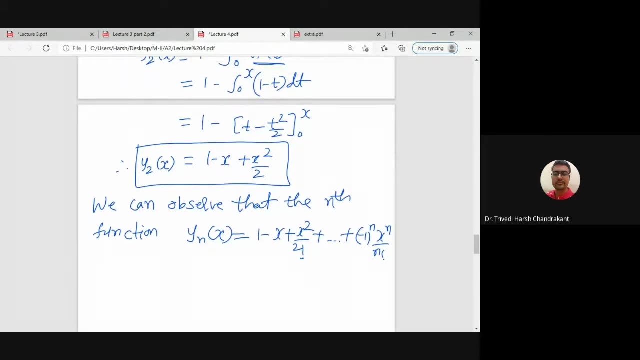 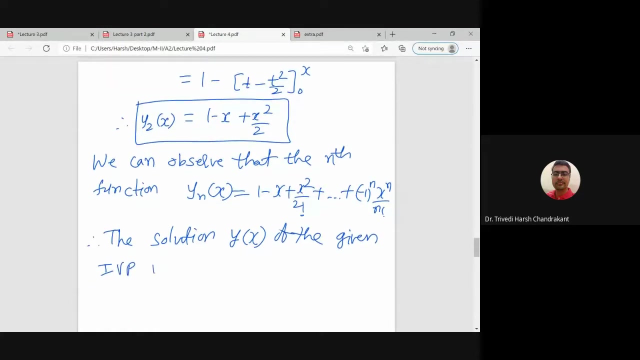 so on plus, so sine is alternating. so that means minus 1 power n, X, power n by n factorial, so this is nth polynomial. so now these polynomials satisfy certain formula. so what will be the solution therefore? the solution yx of the given initial value problem, using the Picard's iterations. 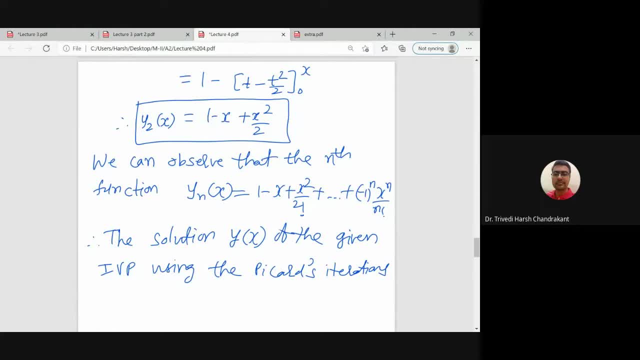 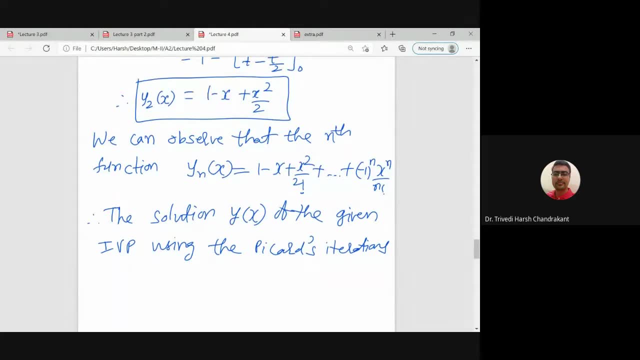 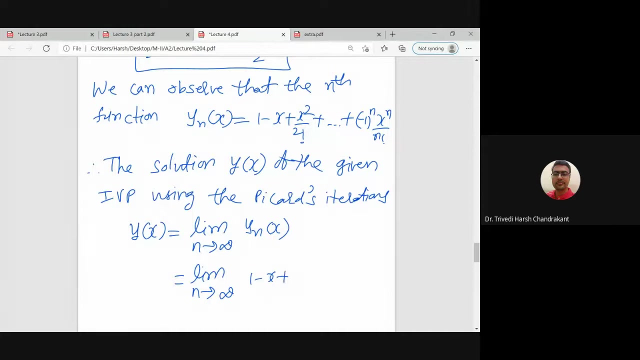 so what are the Picard's iterations? this y naught function, y1 function, y2 function- all these are the Picard's iterations. using that we get the solution yx, which is nothing but the limit of ynx. so it is limit n tends to infinity, tapi to y2. function y n inside x. 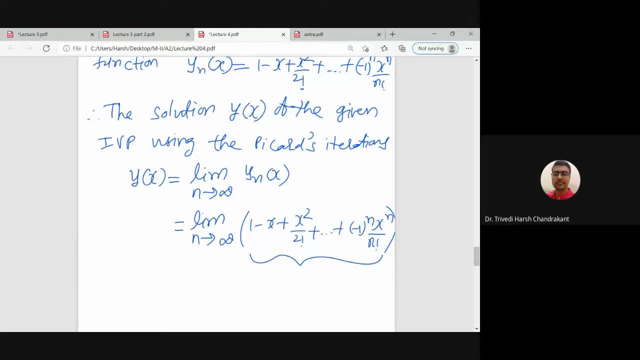 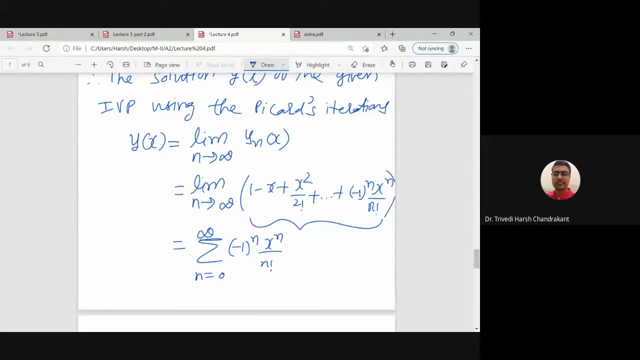 so, if you remember from calculus, this is nth partial sum of certain series and this we can write as a series. n is equals to 0, to infinity minus 1. power n, x, power n upon n. and this series is well known series. it is series of the function e power minus x. 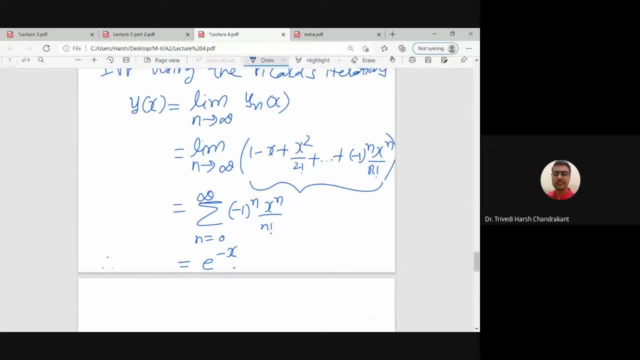 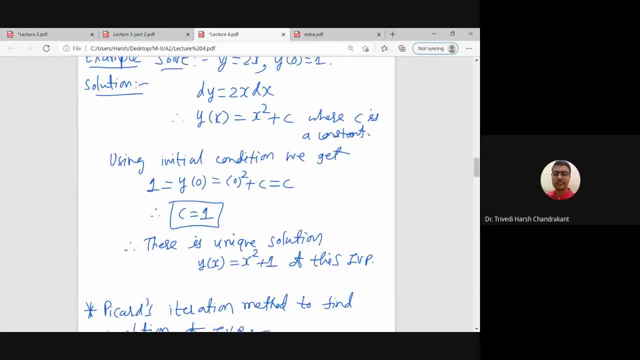 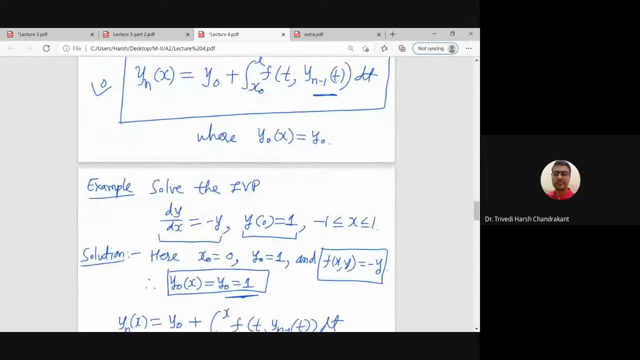 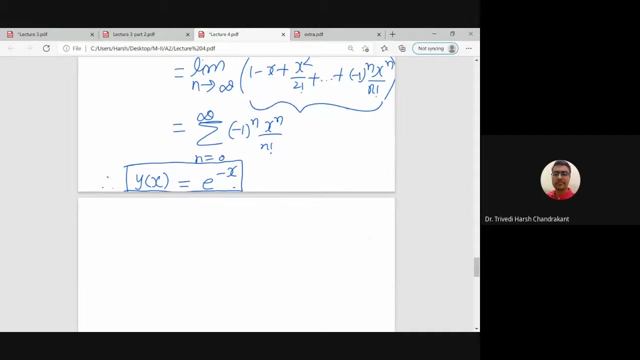 right. so our solution is y x equals to e power minus x and we can see that it satisfies the initial condition. so initial condition is: y 0 is equals to 1, so whenever we substitute x equals to 0 in e power minus x, it will become the value 1. 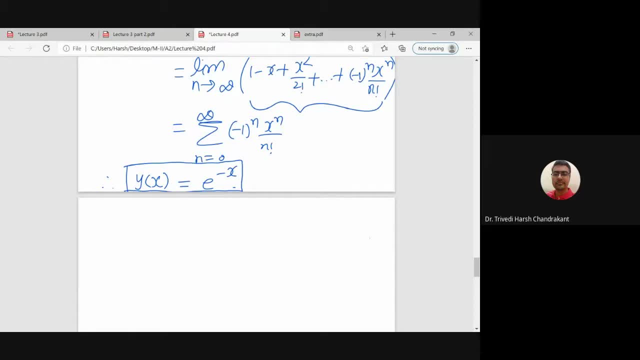 right. so picard's iteration method gives us solution of the given initial value problem, right. so we are not saying it always gives unique solution, but it gives at least one solution. if our function f is good enough, that means it is a continuous function so that we can integrate it. we can find the iterations. 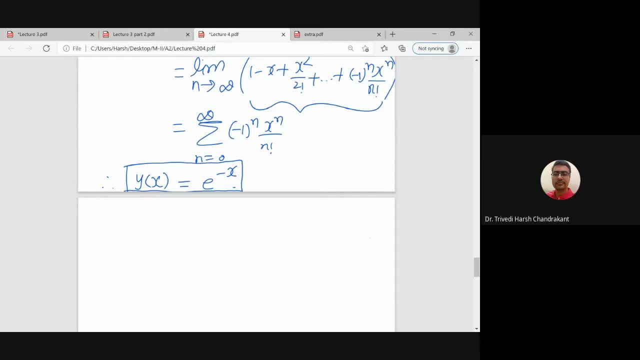 and we can find its limit. that will gives us the function y, which is a solution of this differential equation. you can check that this y- x function satisfies the given differential equation. yeah, so now the next question is how to find the interval. so you said that this iterations, because iterations are defined for. 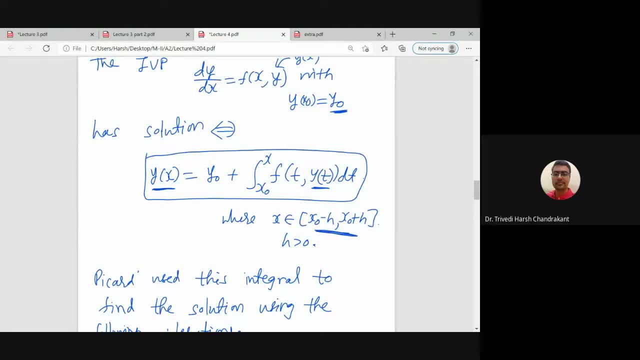 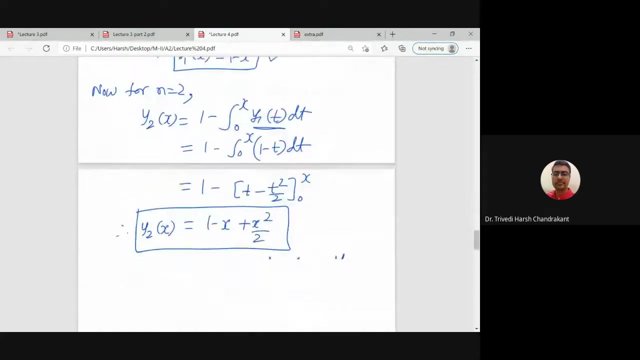 x which is in this closed interval. all right. so that means for which particular interval this function y is defined. so therefore we need to find this possible maximum value of h. that value of H we can estimate using this because iterations. let us see how to find H. so note that the integral y 1 minus y naught, so y 1. we know that y 1. 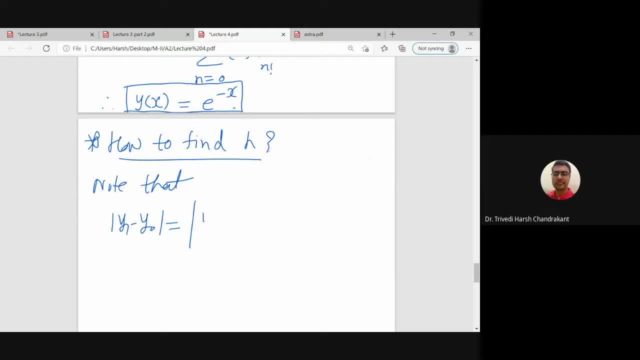 is nothing but y naught, plus integral x naught to the X, F, t, y naught, t, DT and minus the function y naughty naught is y naught constant function. so that will cancel out these two terms and finally we get the integral x naught to. 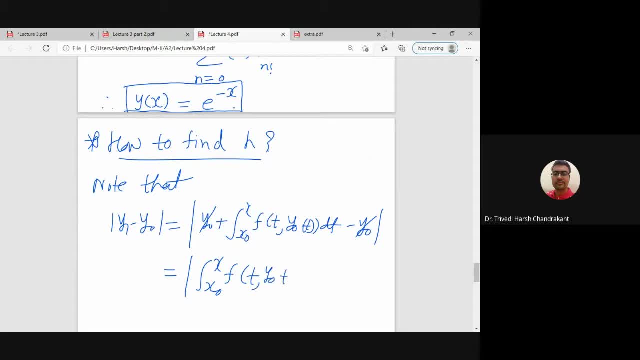 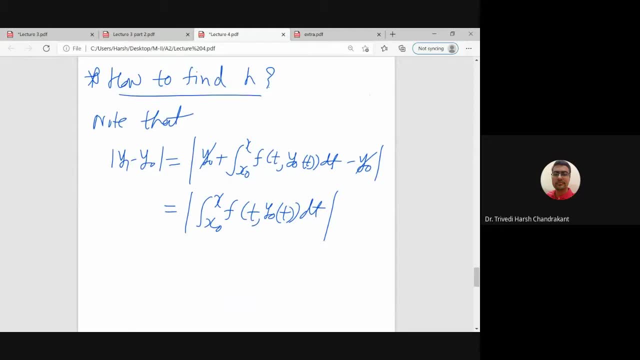 x f of t y naught. y naught, not t dt. so now this quantity. we can see that is less than or equal to length of this. so that means X naught minus X or X minus X naught. modulus value times the modulus value of the function. 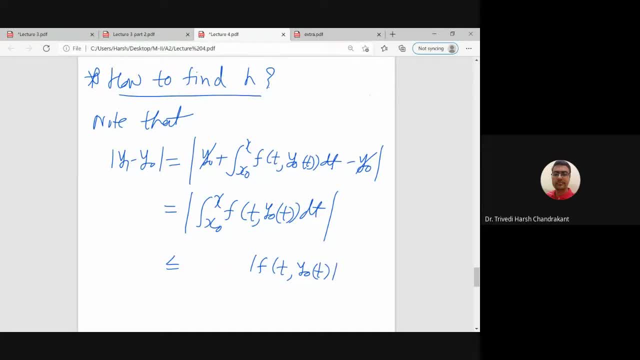 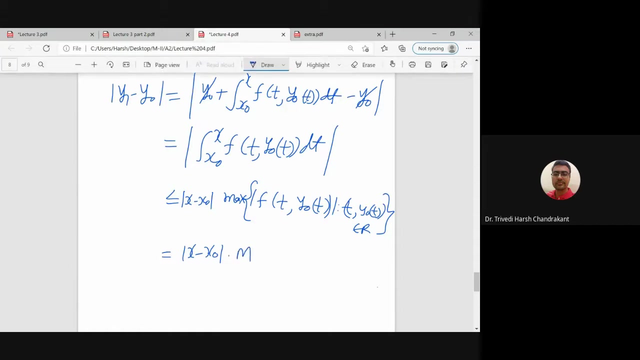 it's maximum value, maximum value of this right. well, T and y naught. T belongs to R, belongs to the rectangle, so that is essentially X minus X naught time right. maximum value. we already noted that. we will denote it by M F- is the given continuous function on the rectangle, then it's maximum value of the. 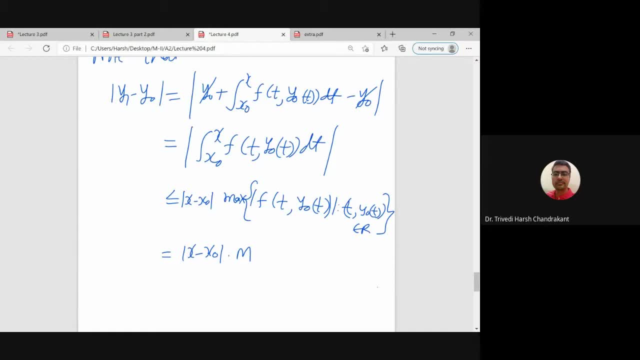 modulus F we will denote by M right, and we know that X minus X naught is H. so this is M times H right. and on the other hand, we know that our, that our potential modulus of Y is X, and then we know that this piece is the. 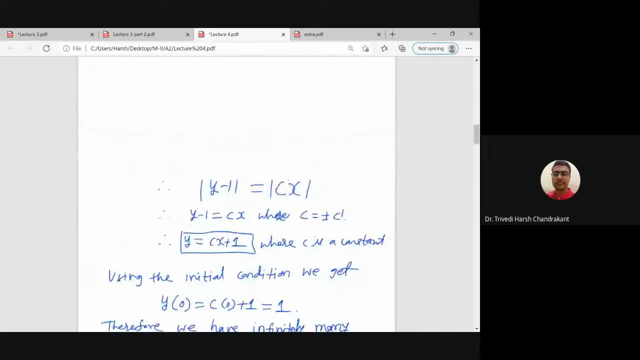 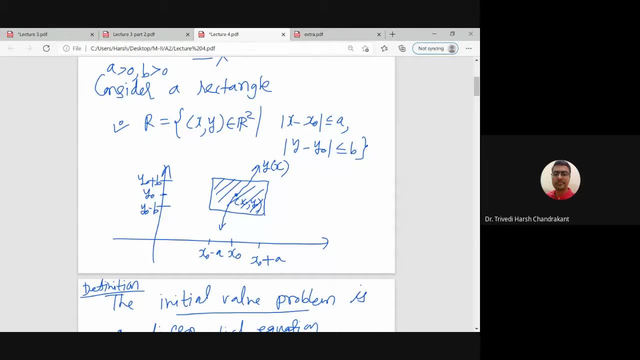 ds slope, and since this, this infinity of planes are non existent, so we can definitely see a negative magnitude that would result in negative coefficient. now what we have to do is double-check all these variable values that we just helped you out. have a needle. so here it tells us that sinceně Reynolds, here it tells us that since 검енно Y also follows the parent series, so it stays 0. and if we plot the125 cela- and now we have to isso, look at it here. and that's our value of the Y. so let us go to the diagram. yeah, so the ourgriff, so the value of Y. so let us go to the diagram F. so let us go to the diagram. yeah, so the our-y naught is our value. sea-нов is between these interval, right? so I belong to y2, y0-b2, y-not plus v. so that means 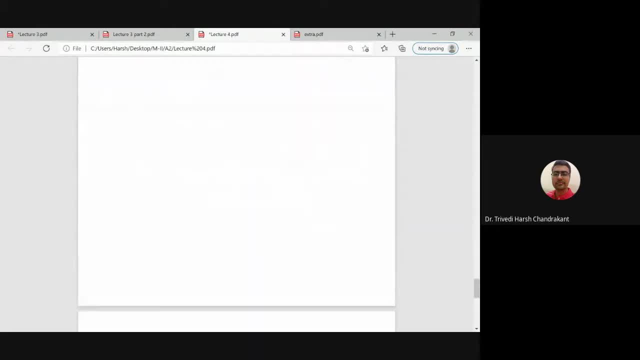 right, less than or equal to b. so this gives us this is less than or equal to b, because y is a element of i naught minus b to i naught plus b. so from this, what condition we got? we got h is less than equals to. 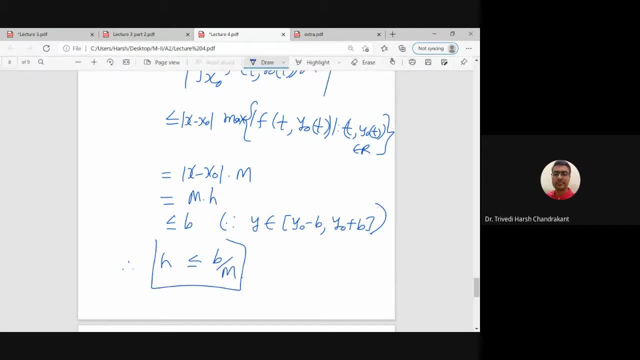 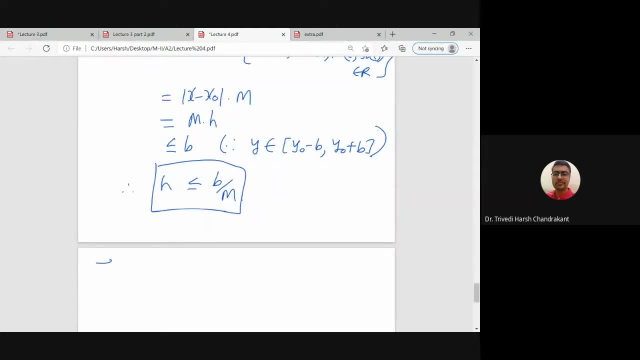 e by m right. in general, we can verify using the nth iteration, that even y n minus y naught is also less than equals to m times x minus x naught, which is equals to m h, which is less than equals to b right. so therefore, in general, we can write: 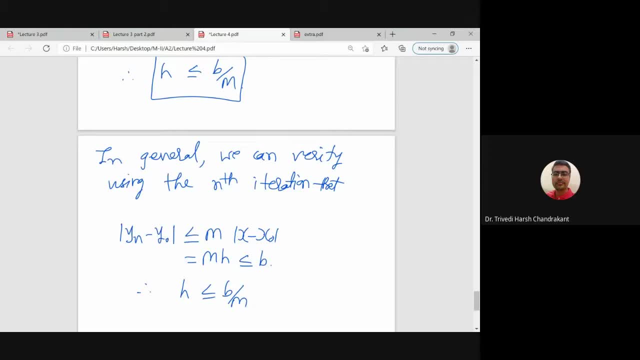 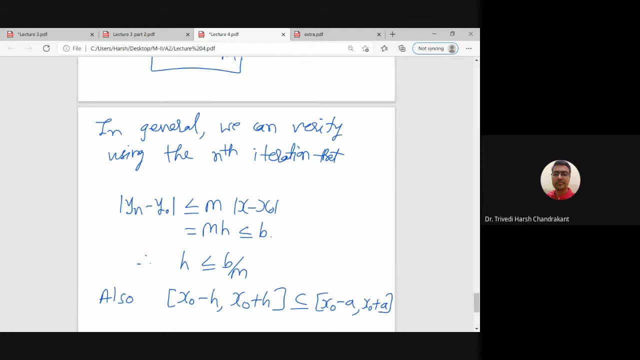 that h is less than equals to b by m, and on the other hand, we already know that the interval x naught minus h to x naught plus h is a subset of the given rectangle. so that means it is x naught minus a to x naught plus a. so therefore, what we get is 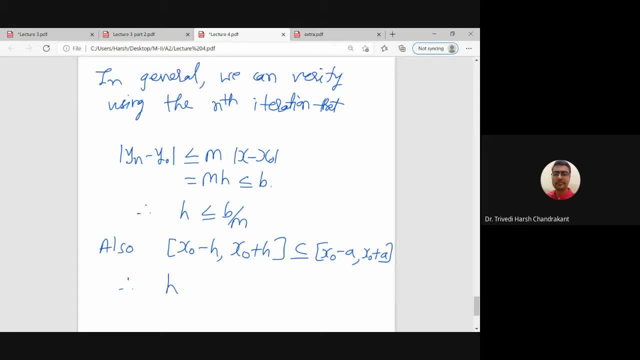 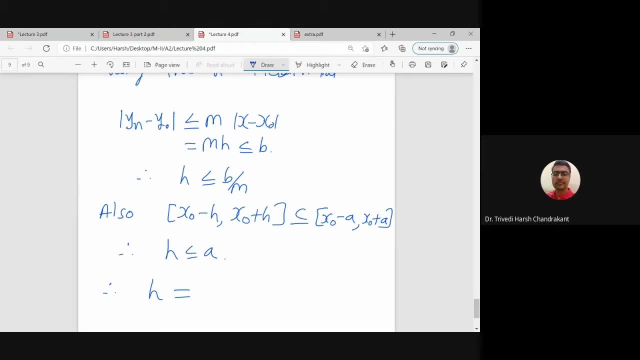 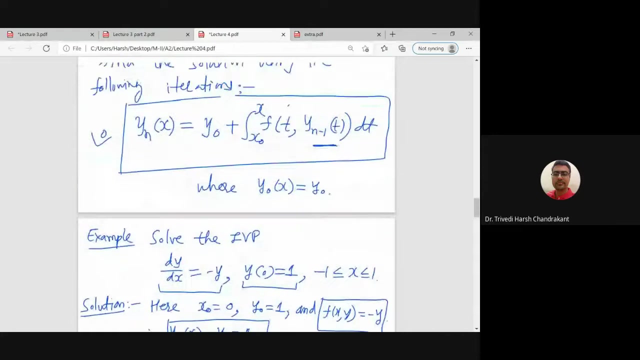 h is also less than equals to a. so this gives us estimate of h is less than equals to a, of H, which is minimum of a and B by M. so why we need to find this? H because the solutions, Y, n because iterations are defined on this particular interval, X naught. 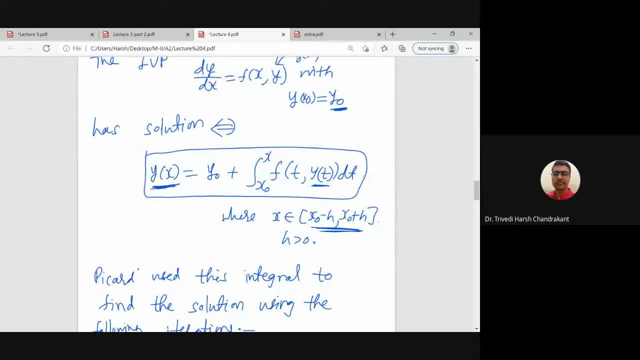 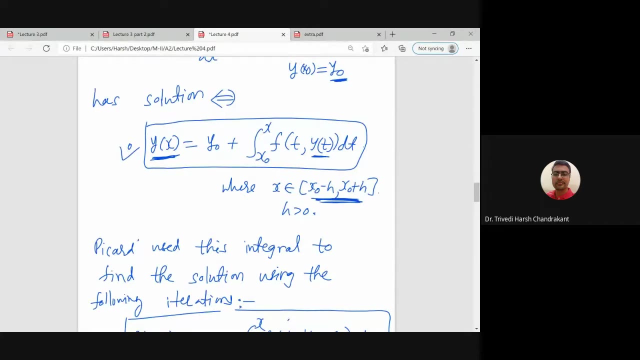 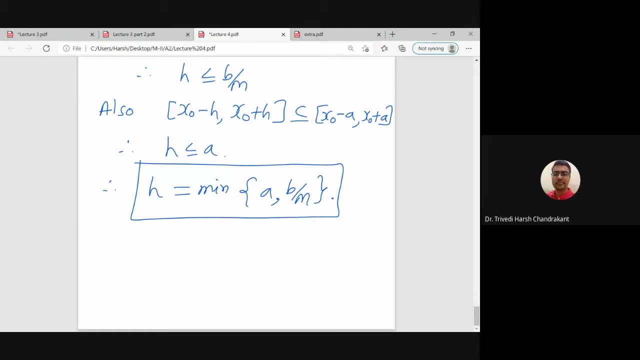 minus H, 2, X naught plus H. this function Y is defined only over this close interval, and this iterations Y, n convert this to the function Y. that means we can find smallest, small enough, interval in terms of H by using this. this formula, over which the function is the function, has the solution. so I 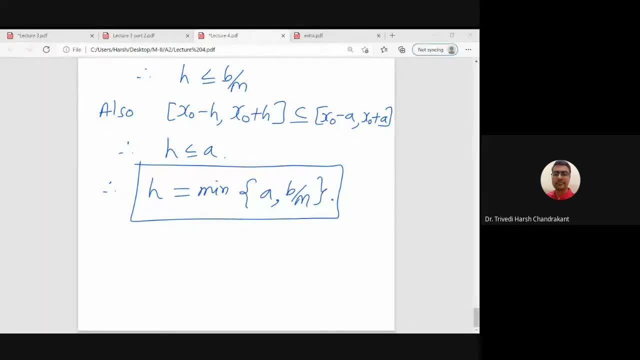 think this should be enough for today lecture, so let me stop the recording.